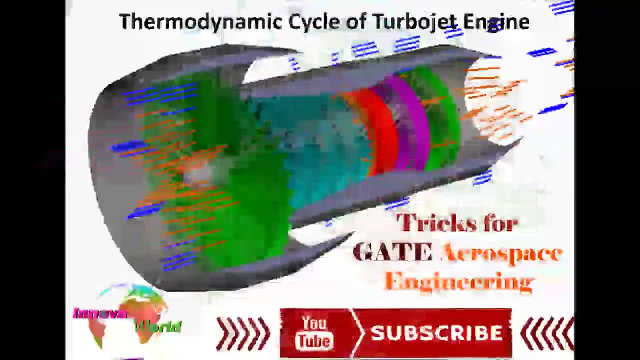 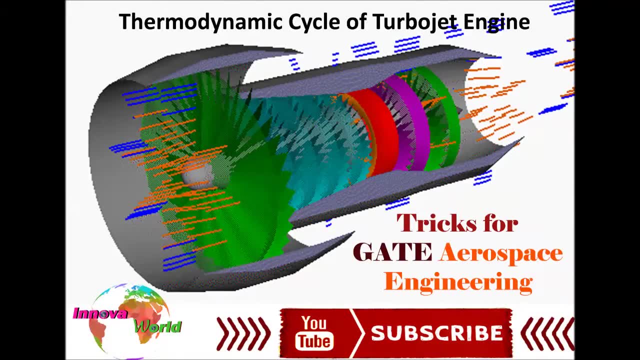 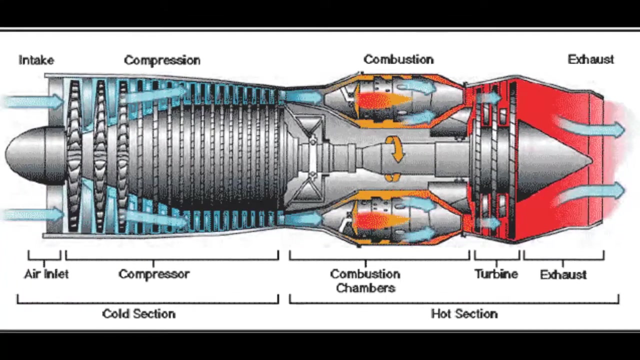 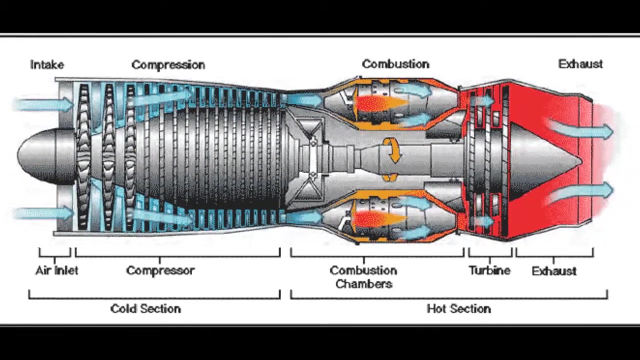 welcome to innova world hello. today's lecture is about thermodynamic cycle for turbojet engine. in this tutorial you can get a tricks how you can easily memorize the efficiency formula for various components in the turbojet engine. turbojet engine can be classified in five sections: air inlet, compressor. 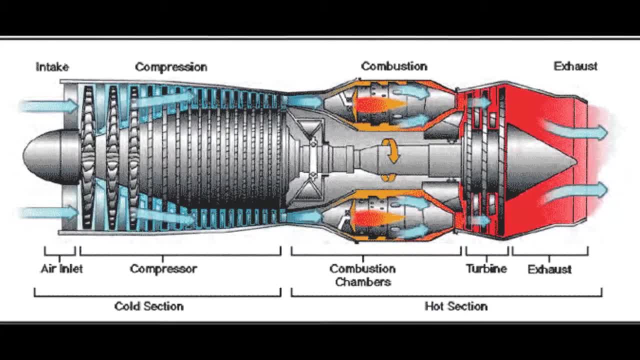 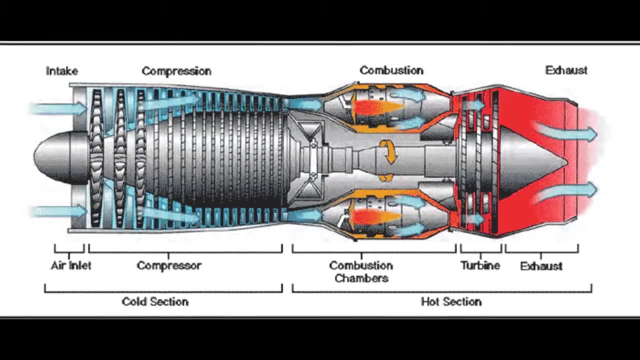 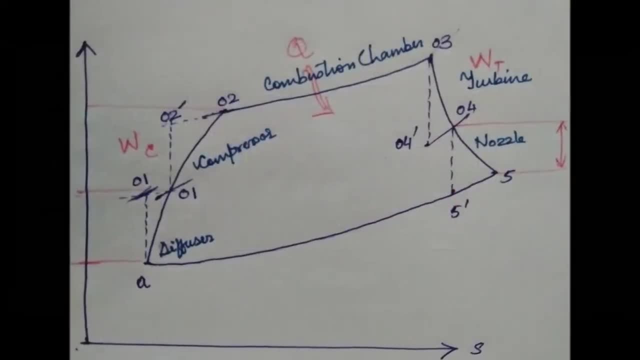 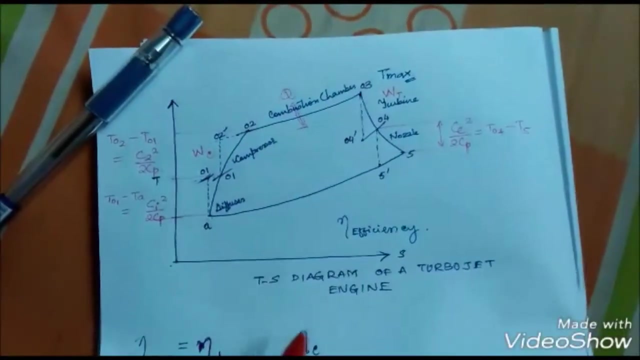 combustion chamber, turbine and exhaust or nozzle in the exit of the combustion chamber will be having the highest peak of the temperature and in case of the compressor there will be the pressure will be the highest peak compared to the other one. ok, so this is our TS diagram of a turbojet engine. so here in the TS, what? 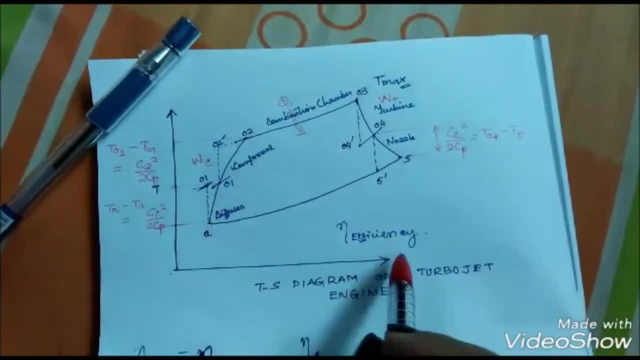 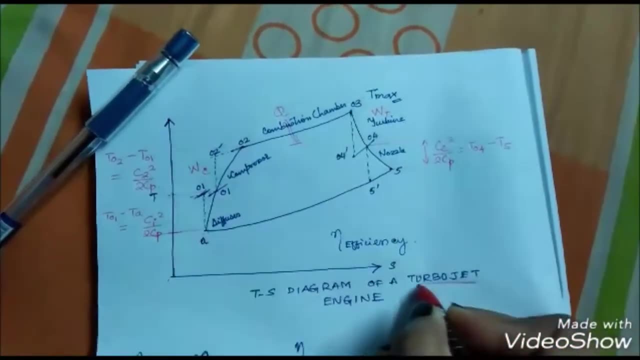 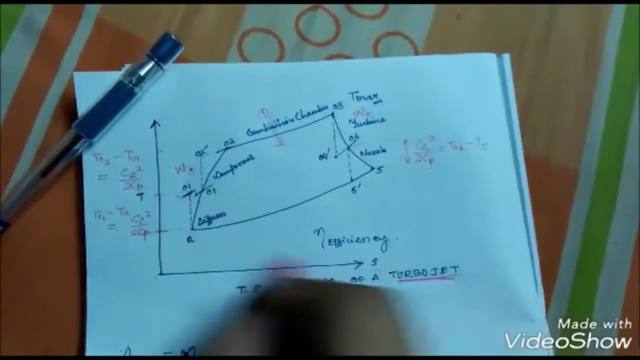 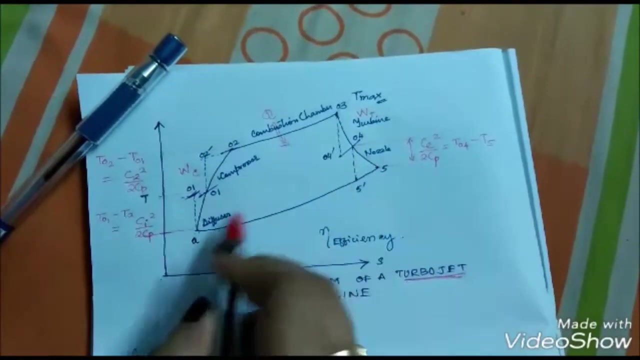 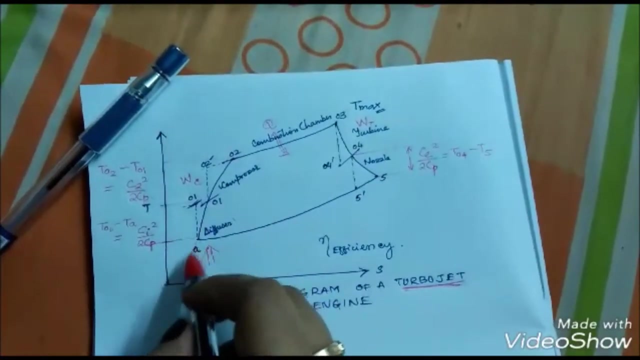 is T. T stands for temperature, S stands for entropy. now here we know, in turbojet engine with it has main, five main components. what are the components? diffuser, compressor, combustion chamber, turbine nozzle. so what the diffuser does, diffuser, it sucks the inlet air. so we can see here, as it sucks the starting point, gradually, what 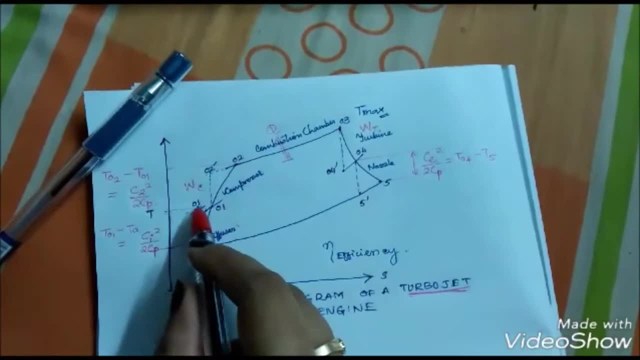 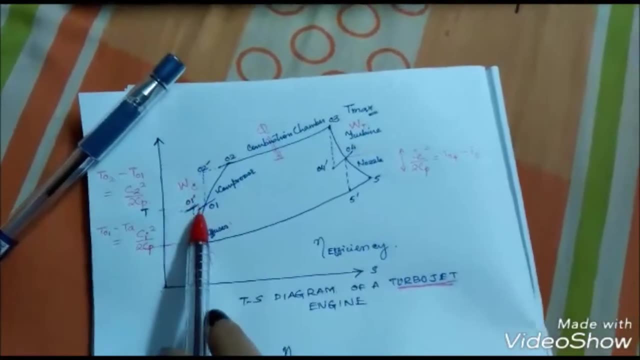 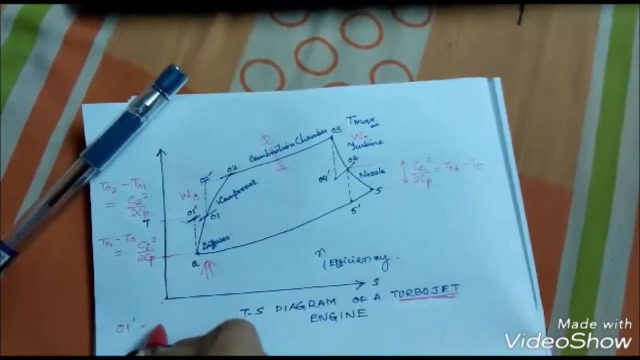 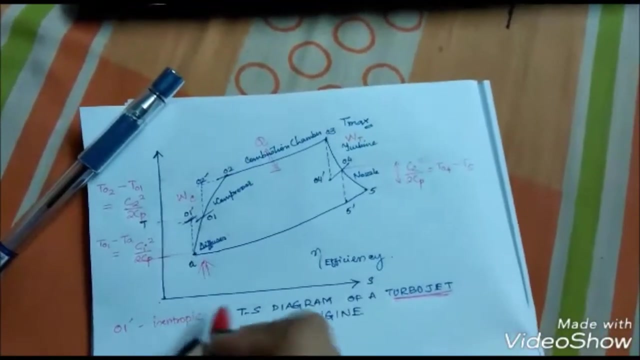 happens this 01 and this 01 dash. so what's the difference between 01 and 01 dash? the 01 dash is the ideal condition, or rather we can say ideal condition- isentropic condition. 01 dash is an isentropic condition or ideal condition. both stand with. 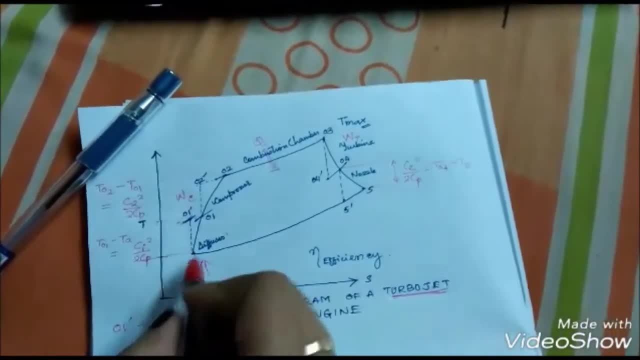 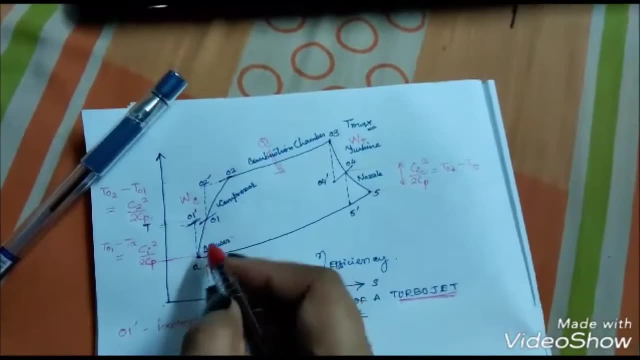 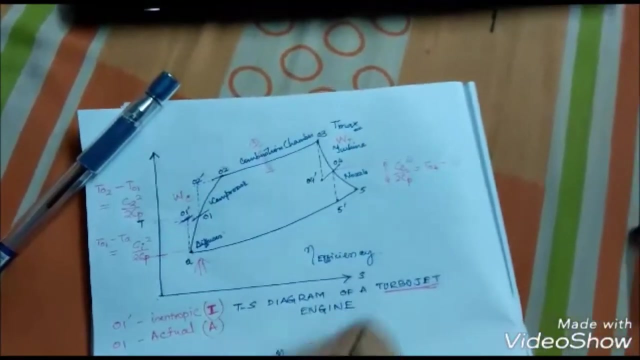 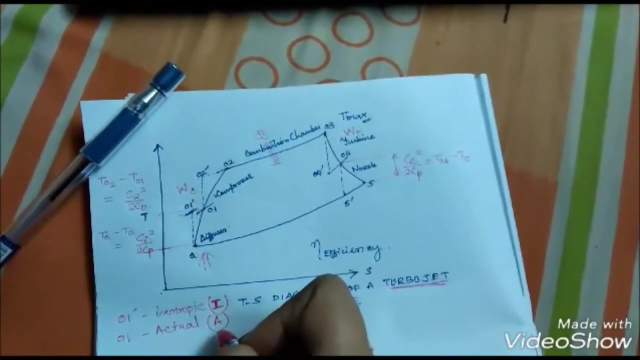 the letter i. this is a way you can remember and the thick line you can see. the thick line going from a to 01 is the actual condition. 01 is an actual condition, or rather you can say as a right now what happens here. so in actually what you see there is, there is some increase in. 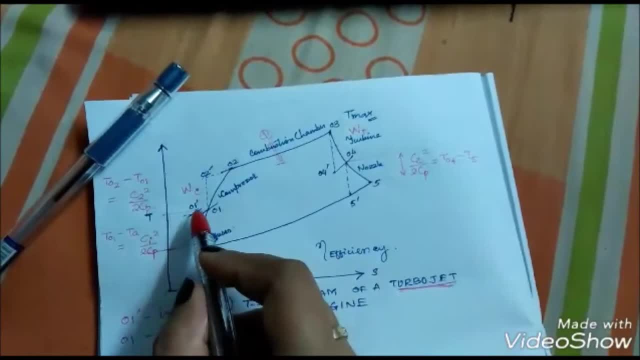 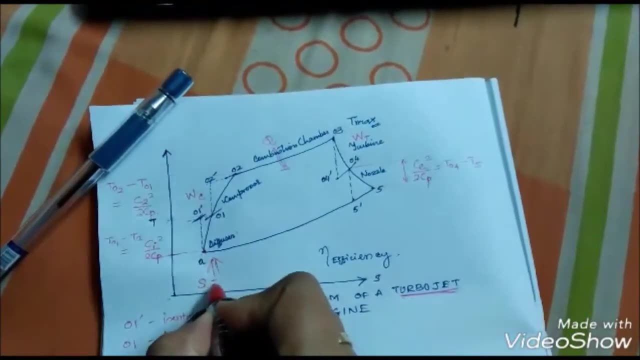 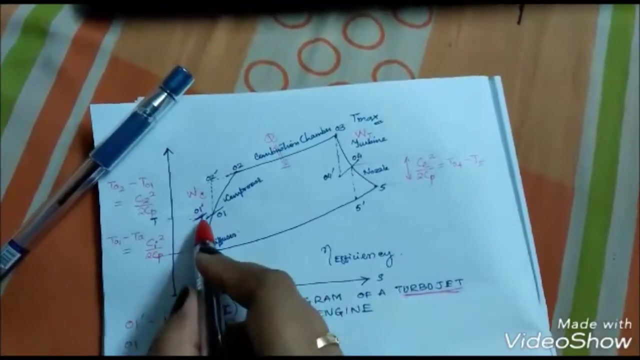 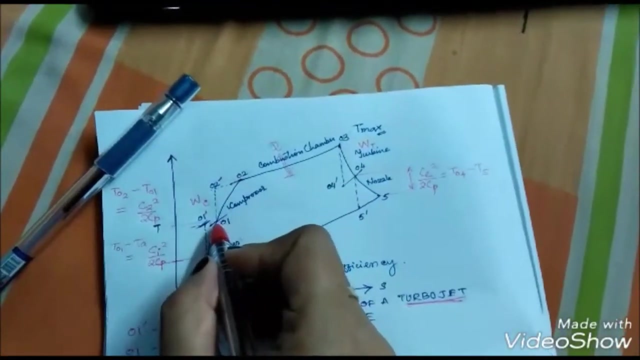 temperature with respect to the entropy. but whereas in isentropic condition what happens? that isentropic condition, that is, s is equals to constant, s is constant and the temperature gradually increase. okay, after it enters in the combustion compressor. this is a. 01 is the entrance of a compressor here. 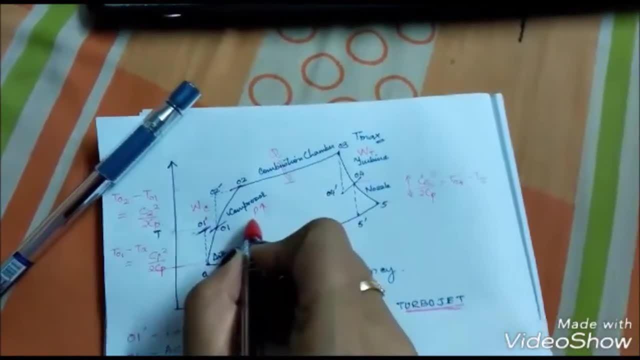 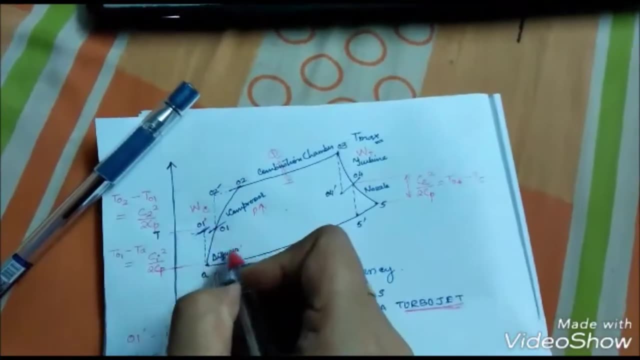 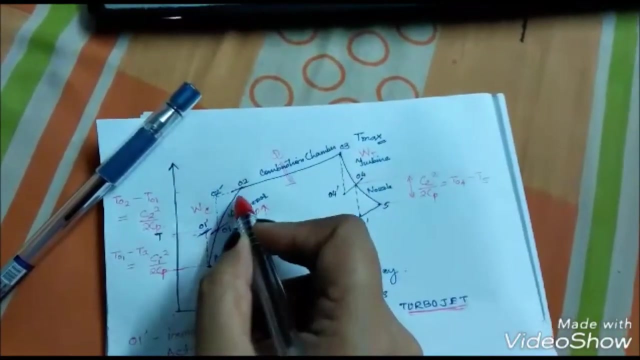 what happens the compressor? the pressure increases, the pressure increases. so 01 to 02. what happens here again? by in by, as the little bit of pressurized air entering the diffuser will enter into compression now. so when it's entering, what happens the compressor? it increase the pressure. 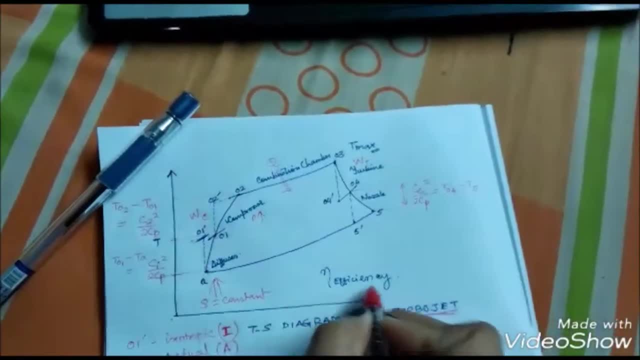 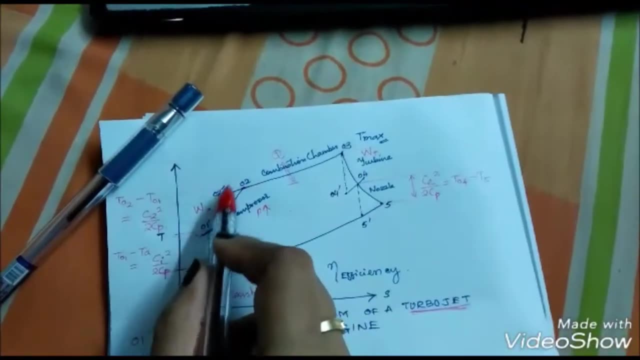 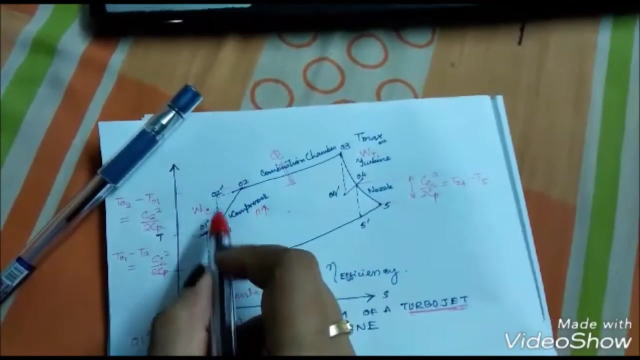 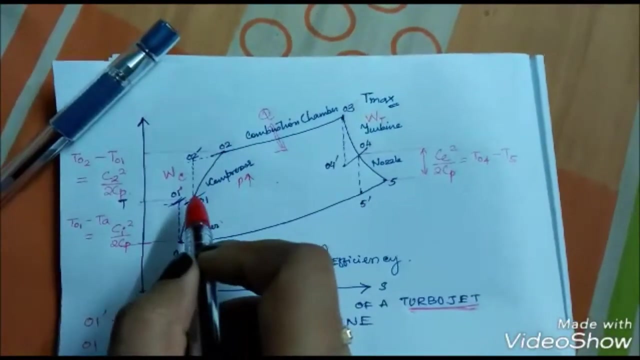 so also it will increase the temperature, as with respect to the entropy. so what happened? here also we have two components, that is, 02 and 0 dash, 02 dash. so here also 01 to 02, what we have. here also we have a straight line with a means of dotted line. you can see by means of dotted line. so what? 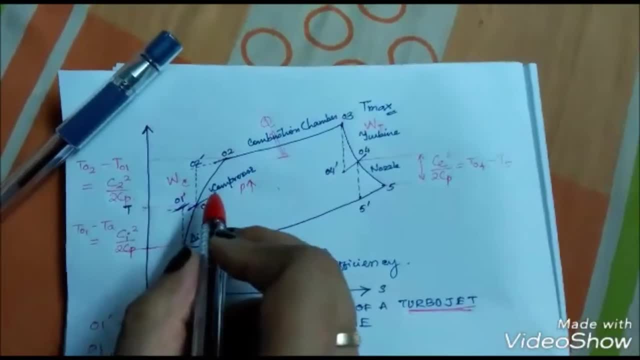 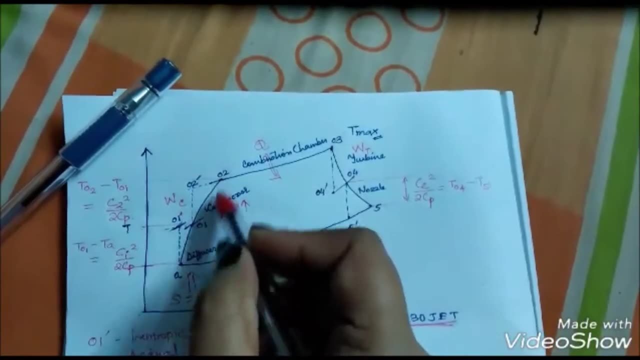 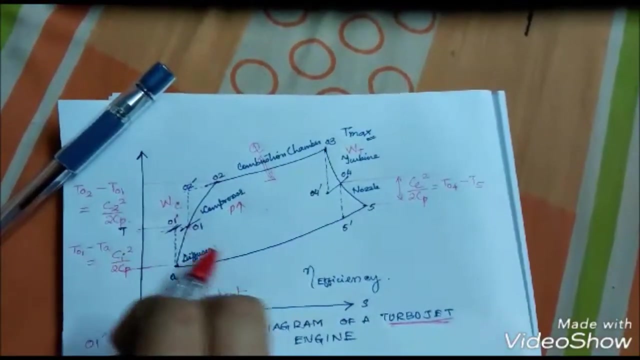 it happens in the dotted line. this is also an isentropic condition, where the isentropic condition is equals to constant, but actual condition: what happens? 0, 1, 2, 0, 2. there is some inclination curvature. that means there is a change- increase in temperature with respect to the entropy. now 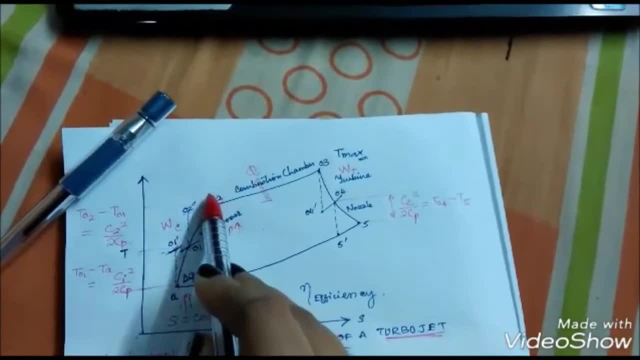 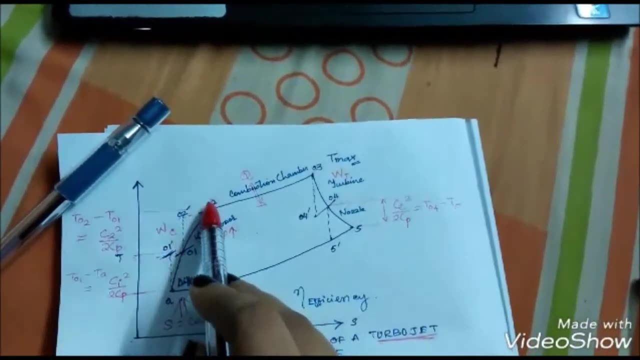 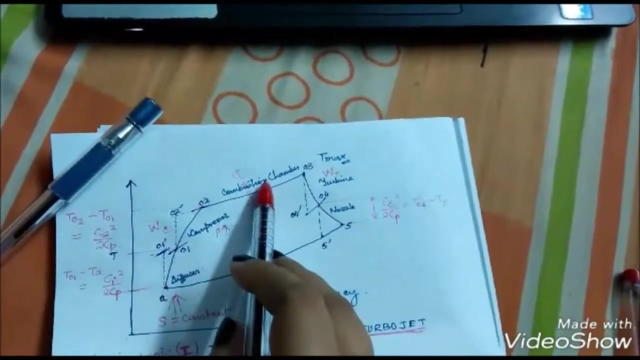 what happens now? after it leaves the car, the pressurized air leaves and enters where combustion chamber- this is the point 2- is an. this is a entrance point of a combustion chamber. so in combustion, the combustion chamber, what happens? there is a combination of the air and fuel mixture. 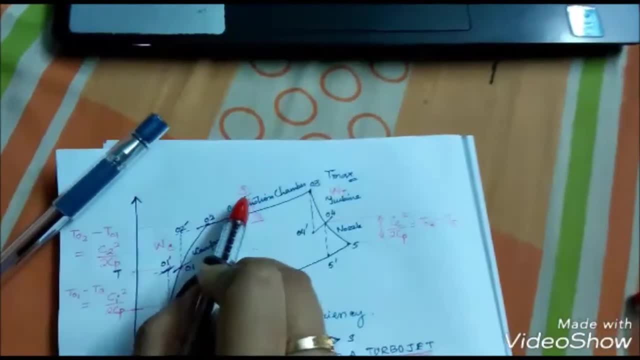 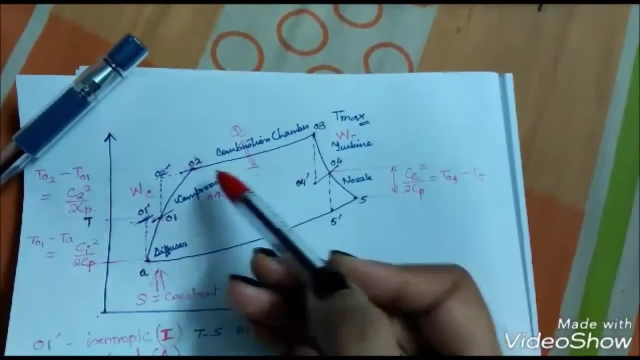 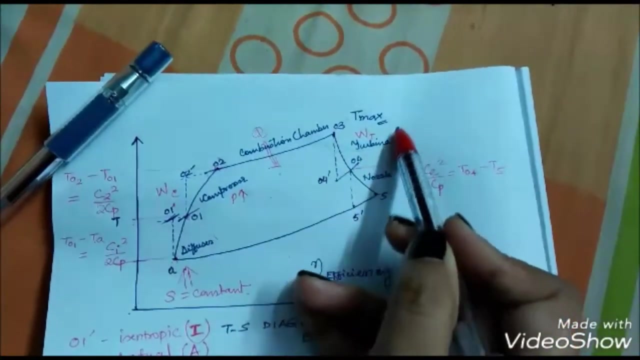 combination of air and fuel mixture, where the heat is added into the system. where the heat is added into the system, so if in the problem, in any other problems they will give you the maximum temperature. so what do you mean by maximum temperature? will occur where? so maximum temperature will occur at the exit of an combustion chamber. 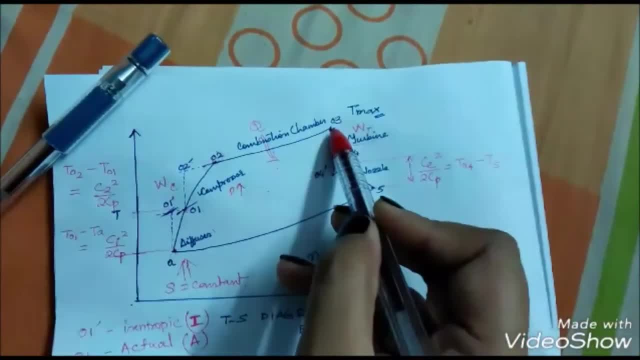 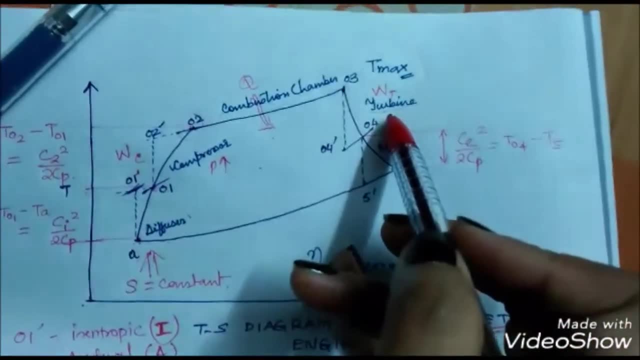 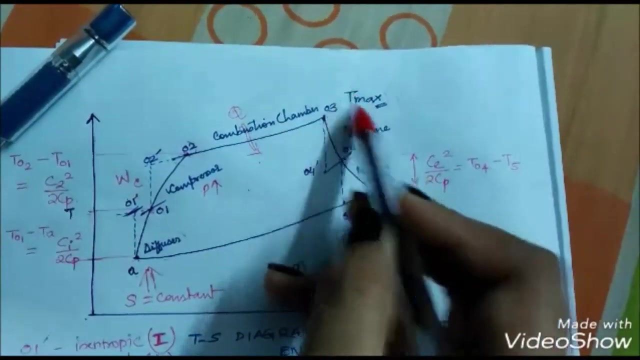 there, at the exit of an combustion chamber, and or rather we can call as an inlet of a turbine, inlet of a turbine or the exit of an combustion chamber, so after that. so this is a point we have of t max, or we can rather cross T naught 3, where we have the maximum temperature. 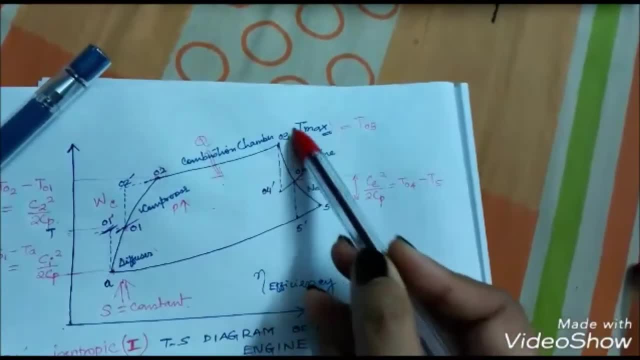 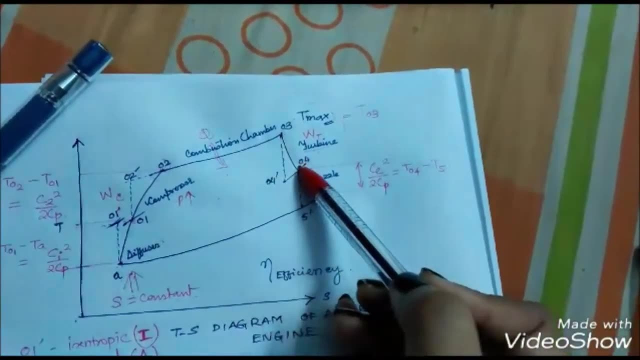 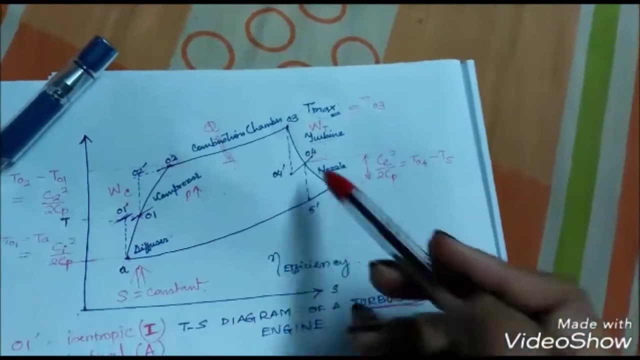 temperature. now, after that, the this air and gas, the high hot gas, where it happens, what happens, it's come out from the turbine. so as it comes out of the turbine we can see that there is an increase. automatically. there is always an increase in entropy, but when it leaves from here, there is. 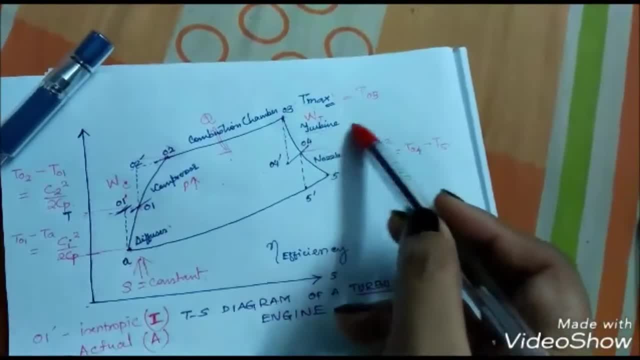 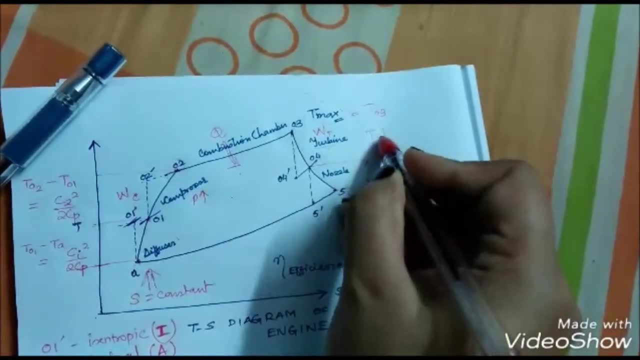 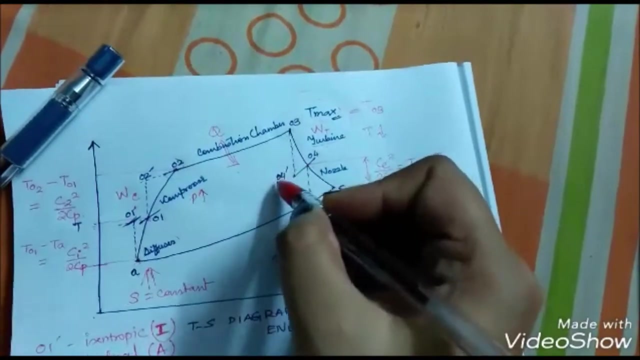 a decrease in temperature. what happens in turbine? there is an increase in entropy, actually, but there is an decrease in temperature. the temperature is gradually decreasing. and here, you see, here also we have a dotted line- that is, this process, that is 0- 4, is an isentropic process where actually 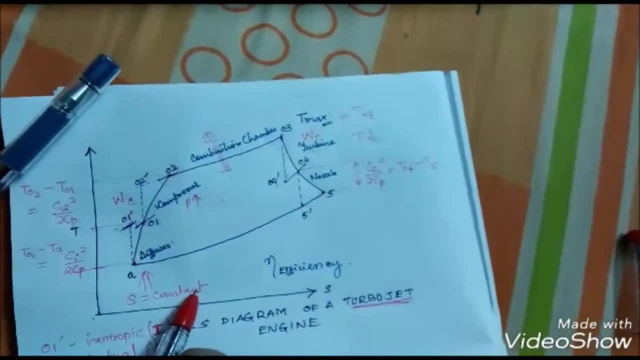 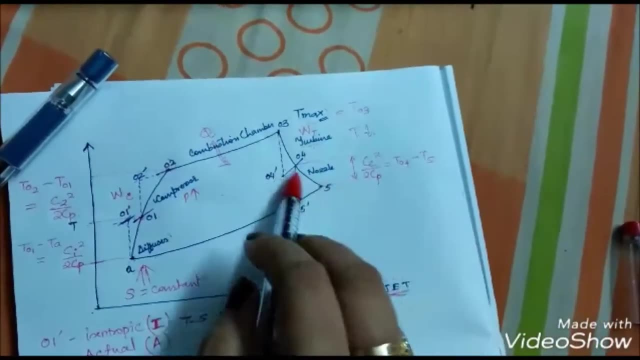 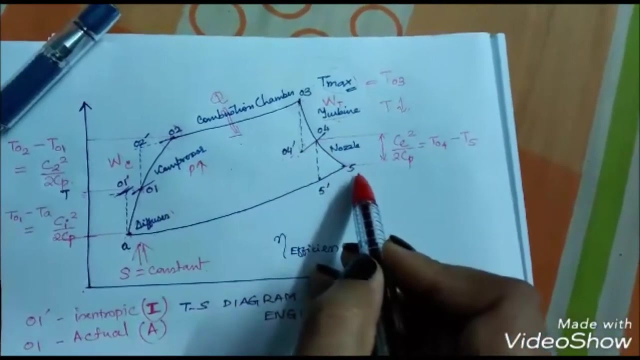 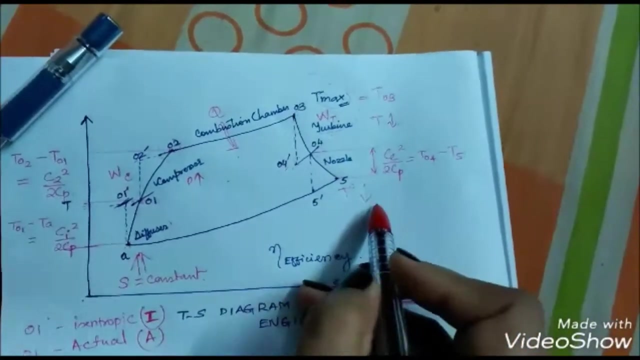 ideally, what happens is is constant, similar process happens that that it comes off from the nozzle. so what is it? we know the function of a nozzle. what happens to increase the velocity. so what happens? here again, as we increase the, as we increase the velocity, the, what happened? the temperature? 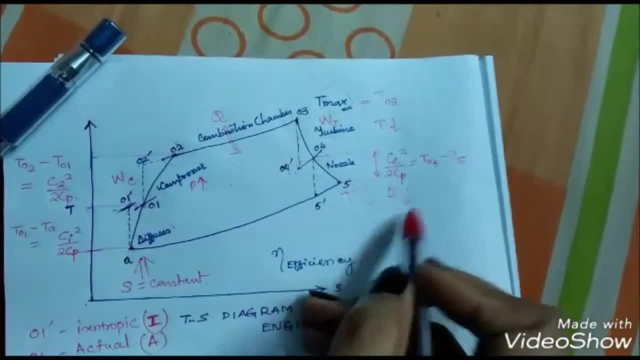 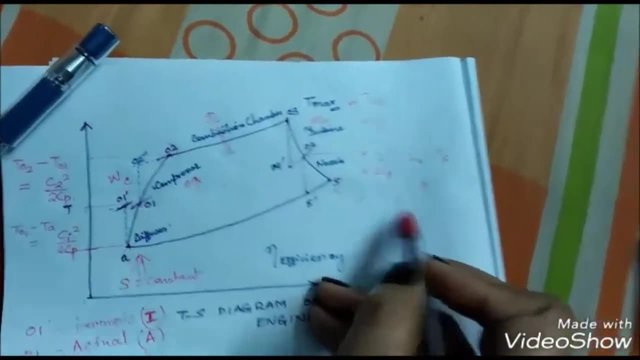 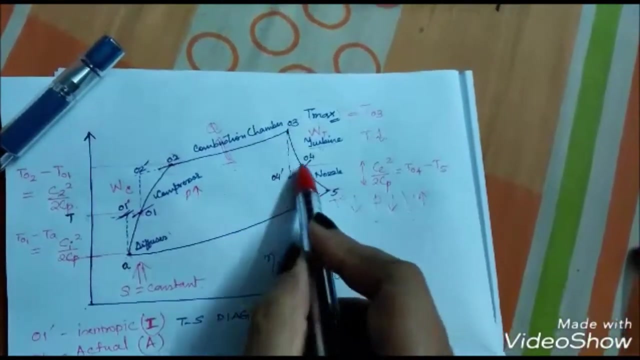 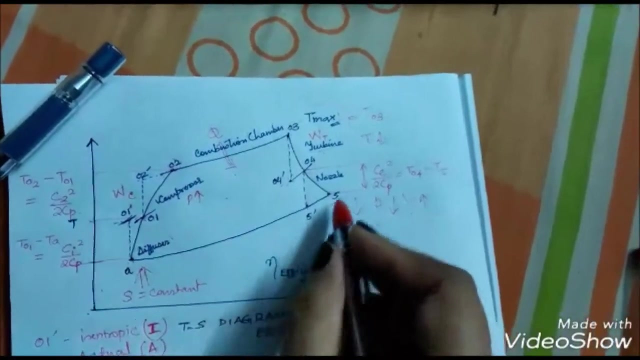 decreases, pressure also decreases to increase the velocity, because the pressure and the velocity are inversely proportional to each other. now here also the same thing: in ideal case or isentropic case, always a dotted line will be a parallel to this temperature line, parallel to this, to the temperature line. so this is a basic, fundamental diagram you should remember and 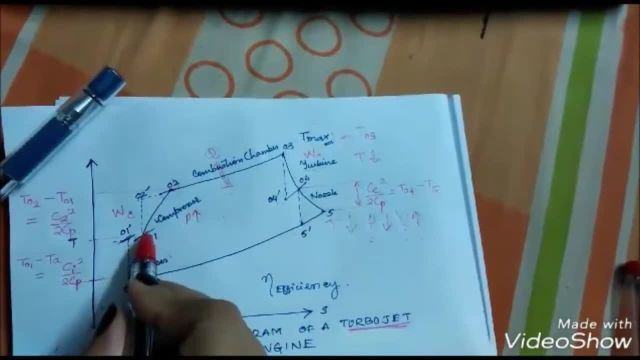 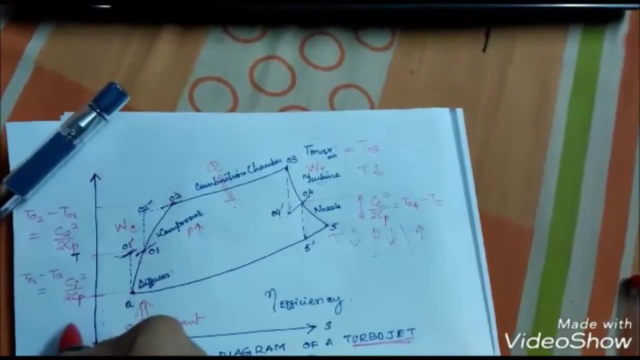 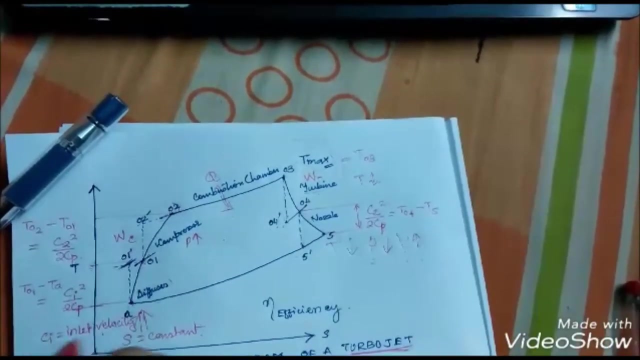 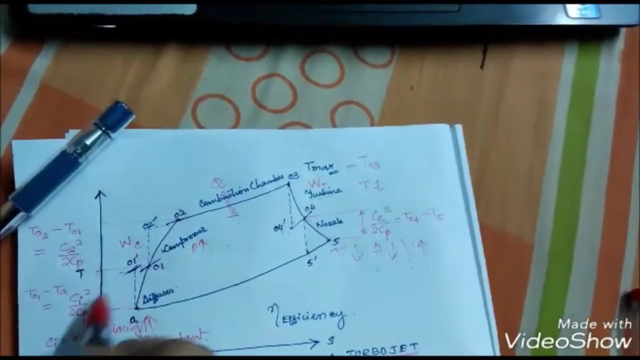 one more point here, from the diffuser to the point. what happens here? this is an inlet velocity. guess that ci. ci is an inlet velocity. okay, so the ci is inlet velocity. the difference of a and zero, one difference of what. this is a point. draw a horizontal line from here, the horizontal. 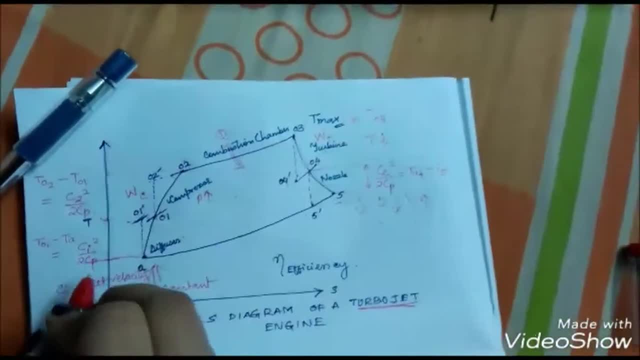 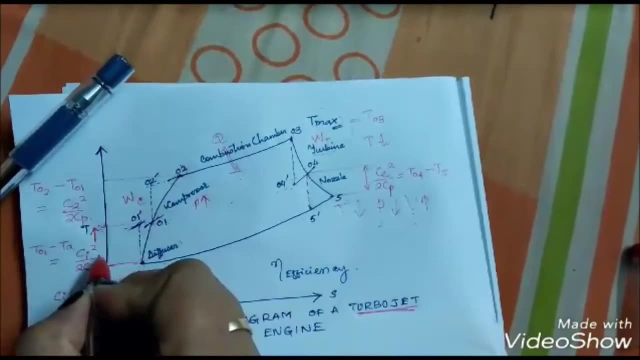 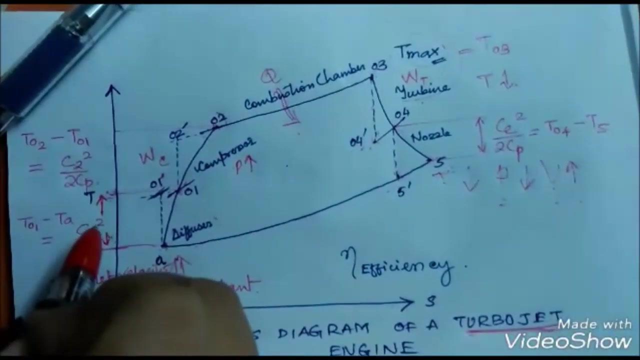 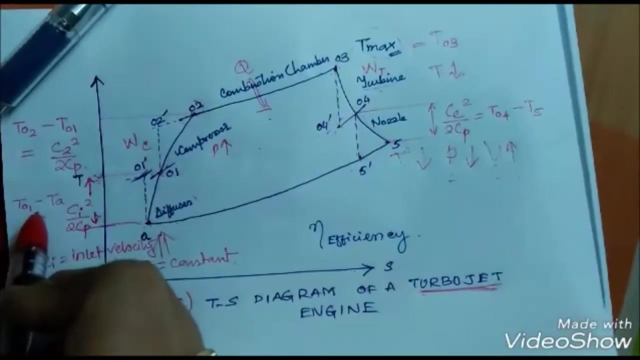 line difference of this two can be expressed by means of ci square by two cp. two square by cp. that is a difference between. so rather we can write: that is: t naught one minus ta equals to ci square by two cp. so in case when there is a requirement, you can apply this value: t naught one. 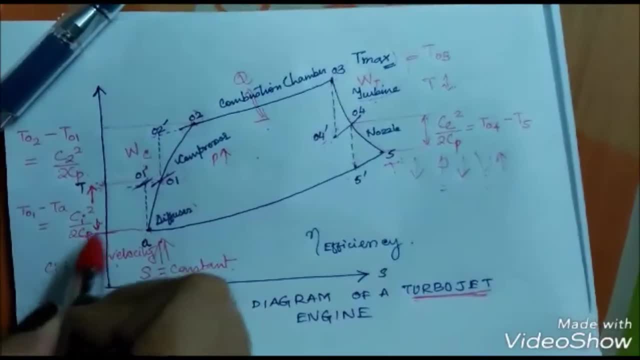 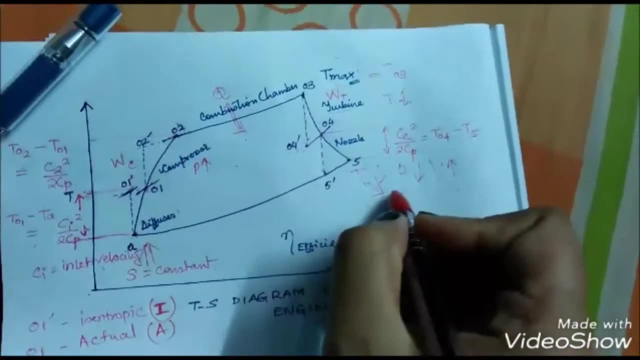 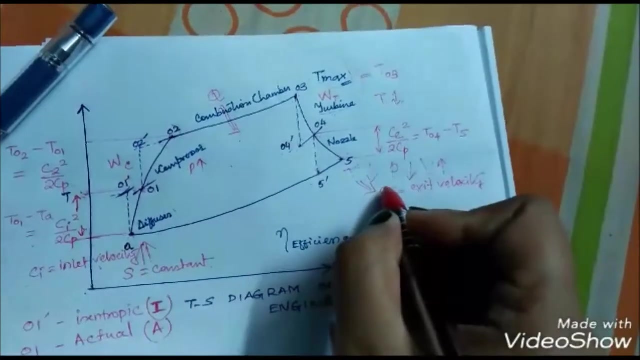 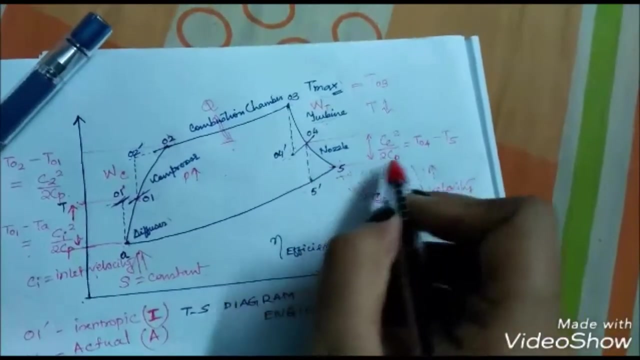 minus TA, the value is CI squared by 2CP. Similarly, what happens in nozzle? The exit gas comes out, In case we name as a exit velocity How we denote it, C suffix E. So here also same thing: The difference between the T04 minus T5, these are the actual value. 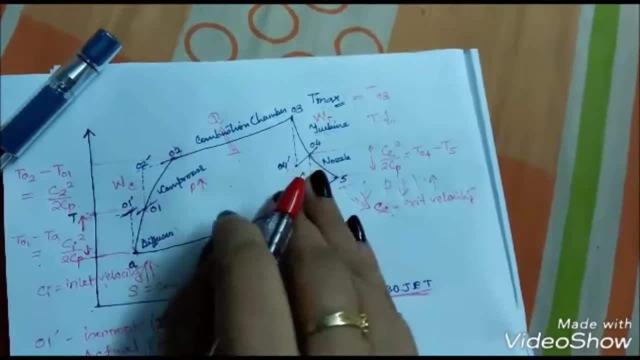 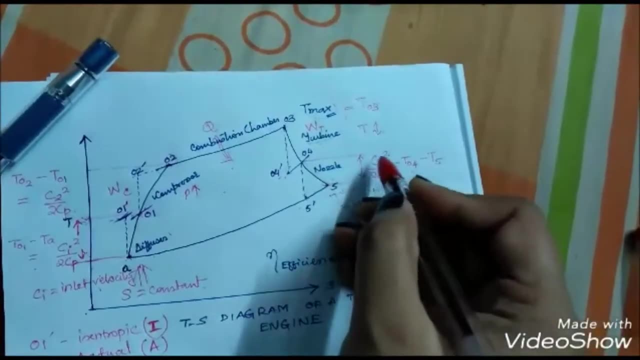 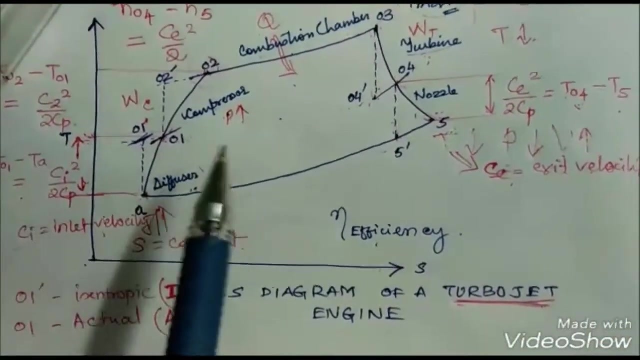 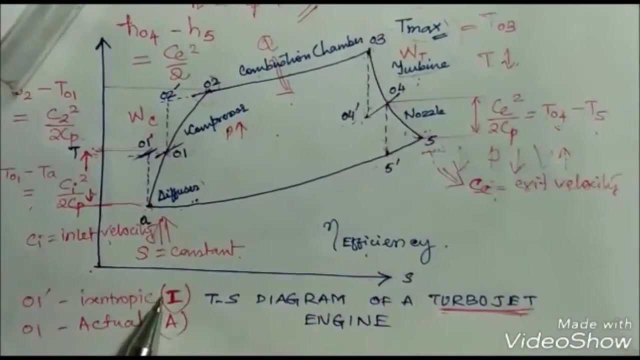 not the isentropic value. We are not calculating any isentropic value. We are only calculating the actual value, That is, T04 minus T5, the difference gives us CE squared by 2CP, Efficiency of an diffuser, compressor, turbine and nozzle How they are interrelated using their isentropic. 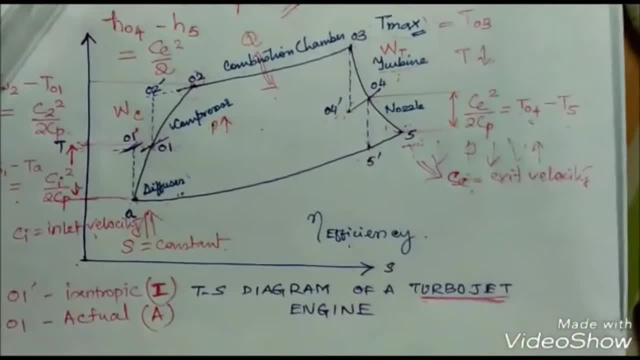 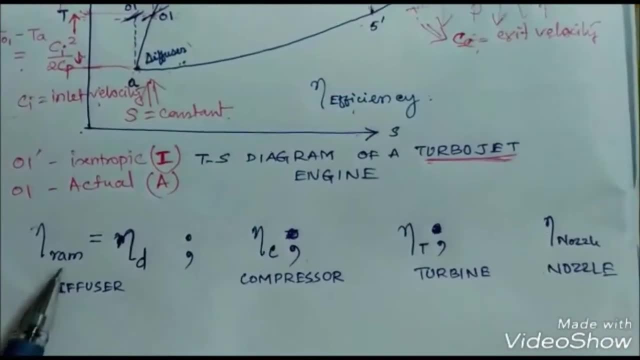 and actual relation Here. in exam point of view, you can easily remember the difference between the two values. So here also same thing: The exit gas comes out. The exit gas comes out. Remember by remembering this dynamic. now we are talking. 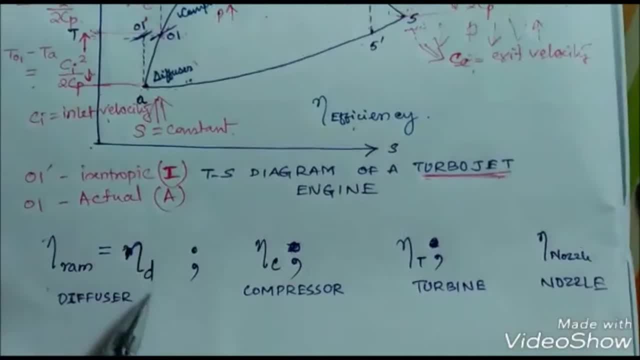 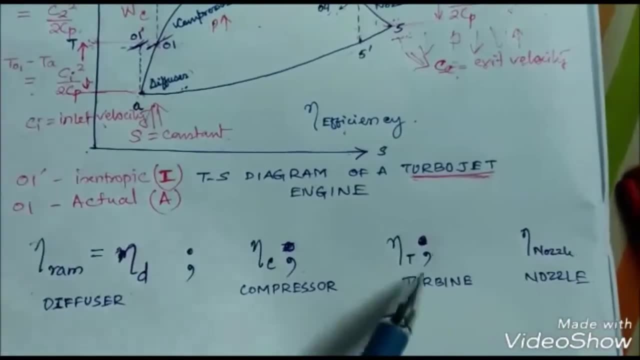 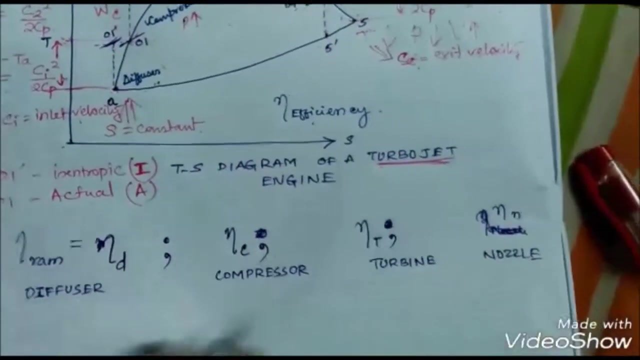 about this main efficiency, that is, the ram efficiency, or diffuser efficiency, can be denoted by the letter eta d, Compressor efficiency, eta c, Turbine efficiency, eta t And nozzle efficiency, eta n, Eta n. So now how you can remember this techniques. 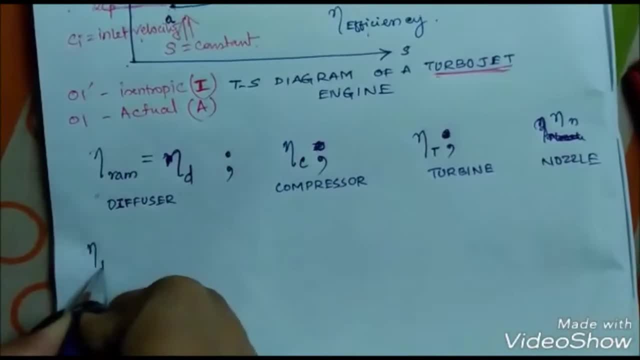 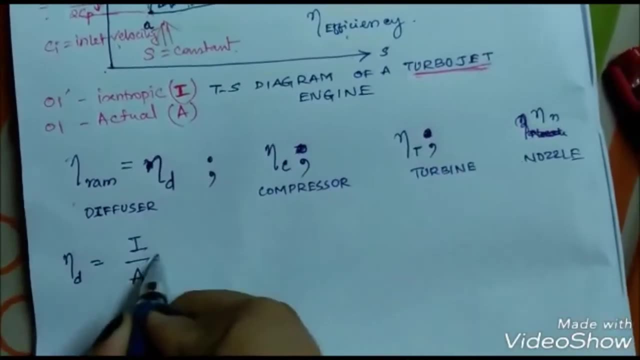 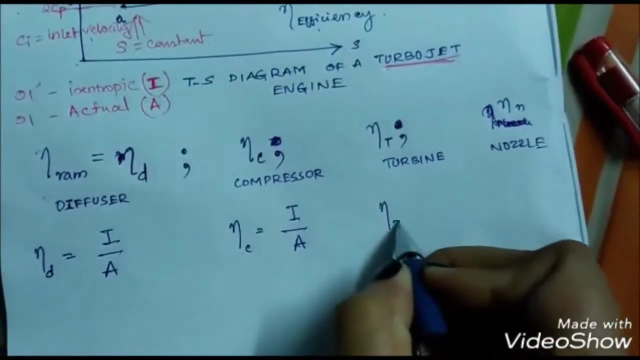 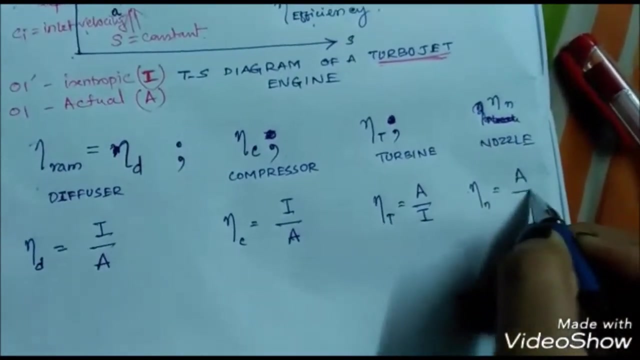 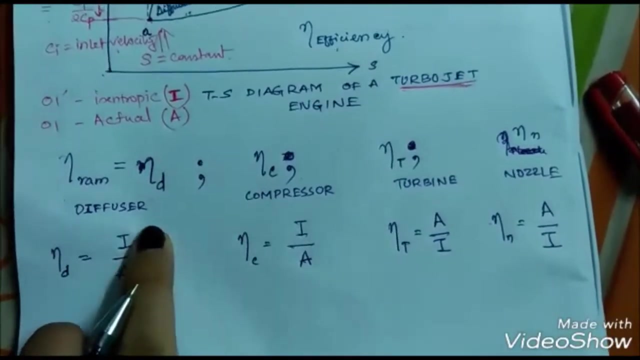 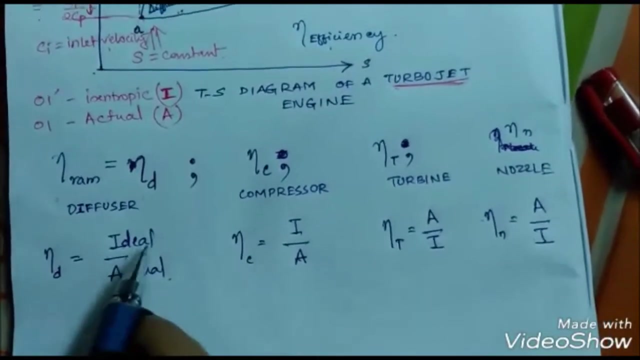 Remember this: efficiency. Eta D is nothing but the ideal by actual. Here, Eta C is also ideal by actual. Eta T is actual by ideal. Eta N is actual by ideal. Now, what does it mean, ideal I by A? I by A is ideal by actual Right. So what is mean by ideal? Nothing but the isentropic relation. 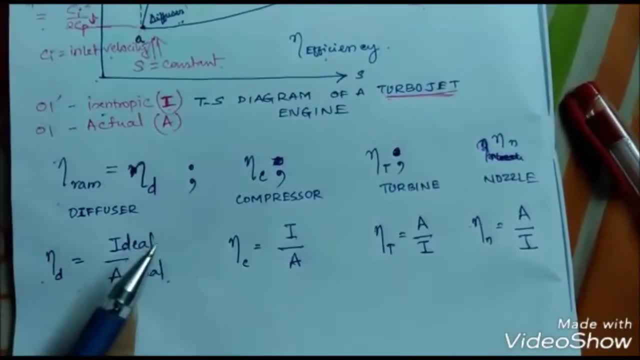 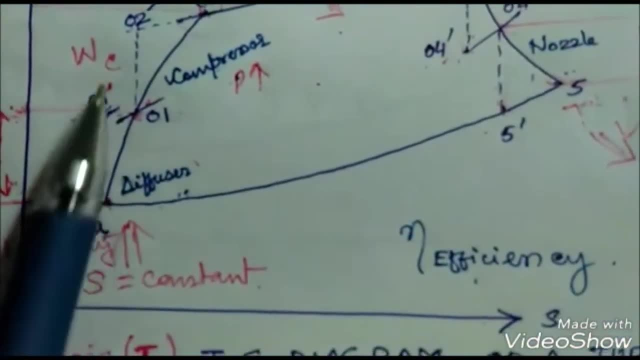 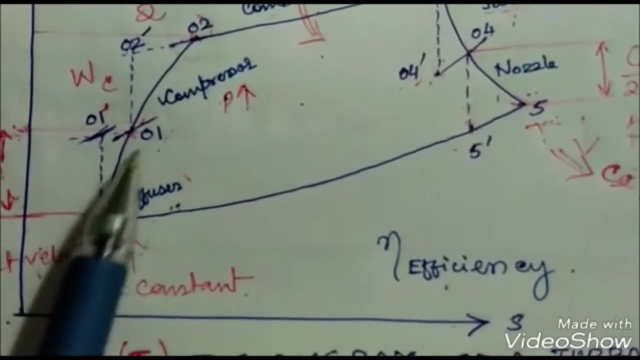 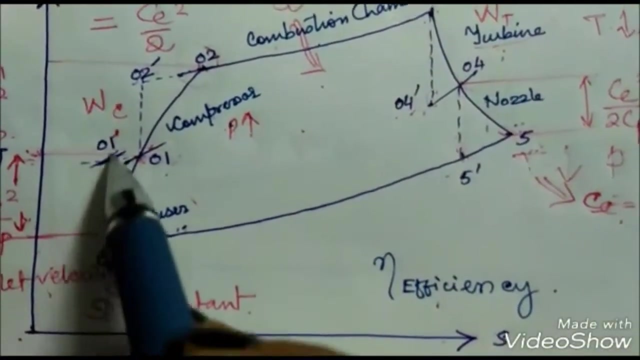 Now you see the diffuser, Now we focus about the diffuser. Now see the diffuser correctly. What we have is point A and 0, 1.. So So A is a, what is a point? A and 0, 1 is the actual point. and A and 0, 1 is the ideal point or isentropic point. 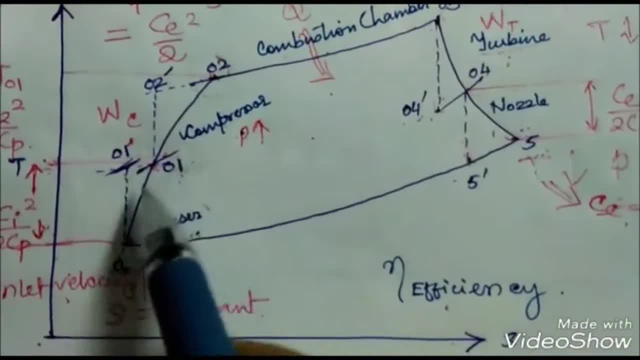 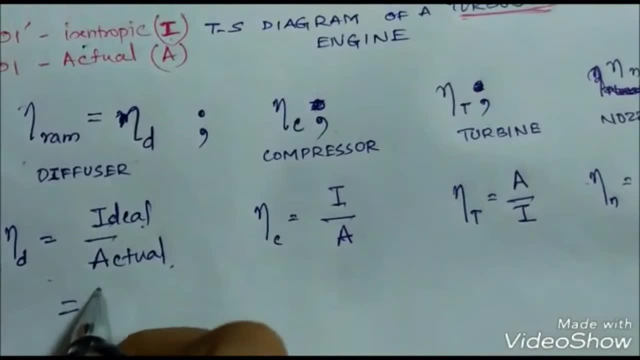 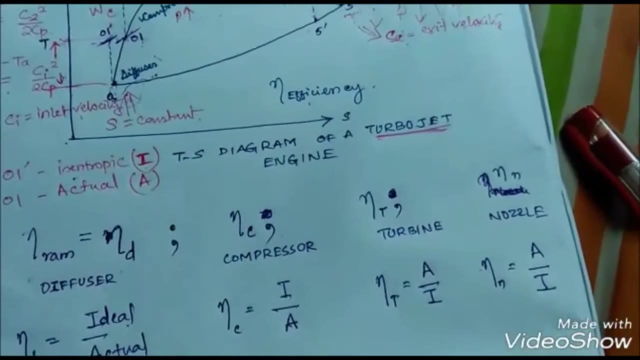 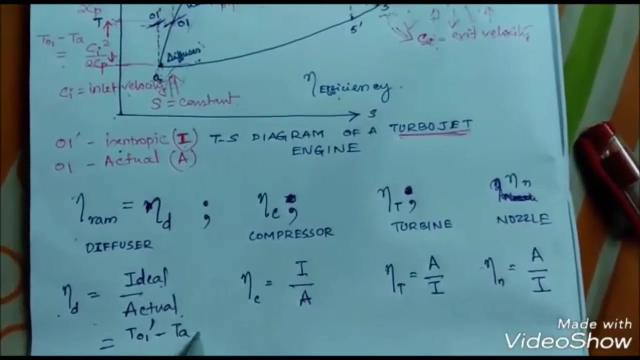 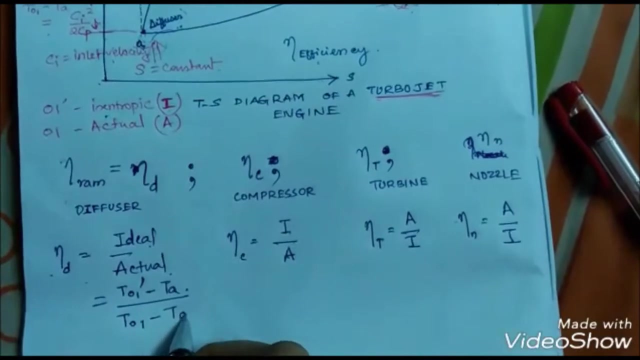 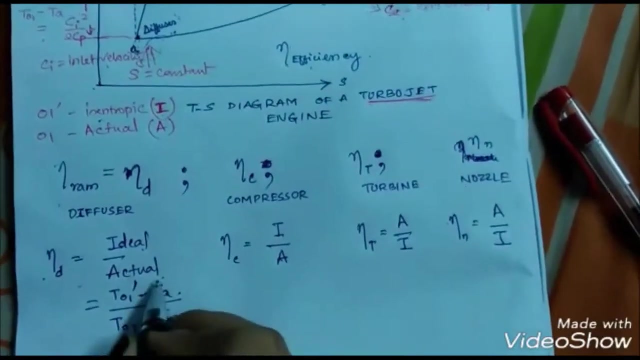 Now who is higher in the temperature? 0, 1 is in the higher, So what we will write is ideal. So here, 0, T01 dash, T01 dash minus TA, divided by T01 minus TA, because we know 0, 1 minus TA, T01 minus TA is an ideal condition. 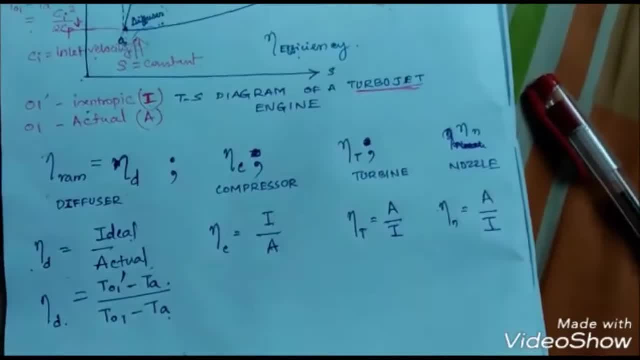 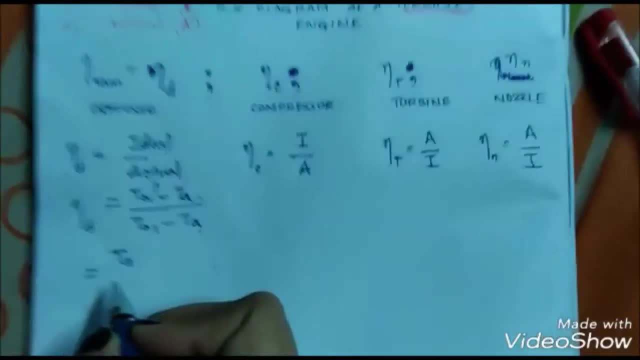 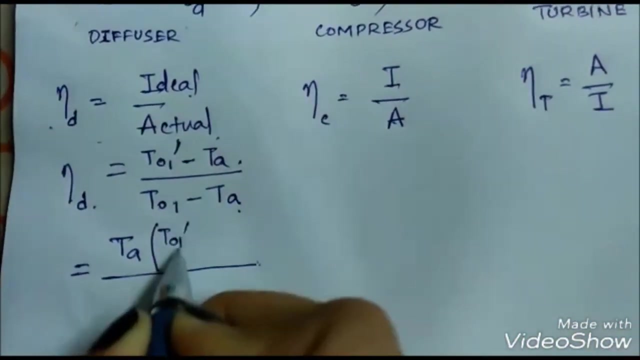 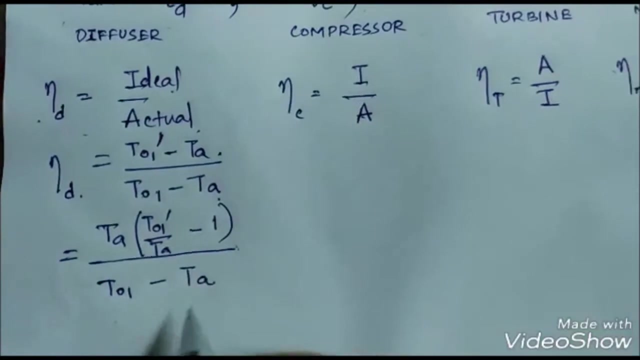 So 0. This is D. Now let me take TA common outside. Now let me take TA common outside. What we will get? T01 dash by TA minus 1.. Here, T01 minus TA. Let it be like that: 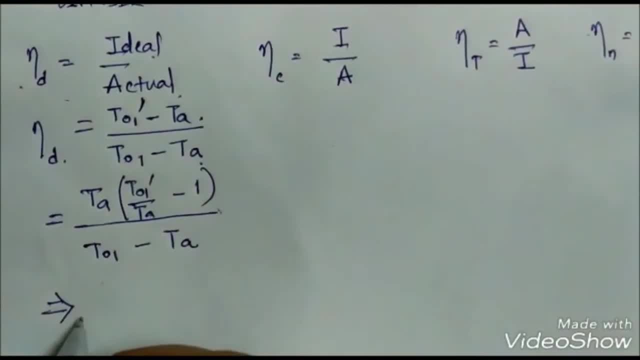 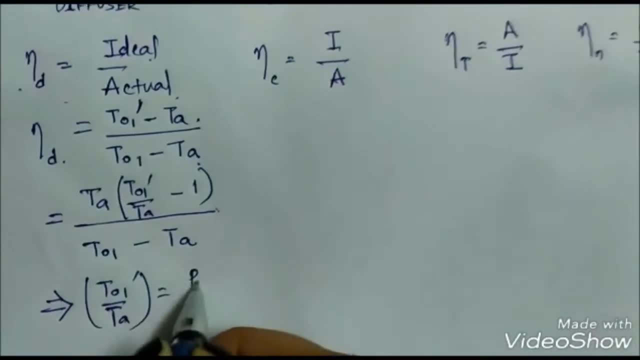 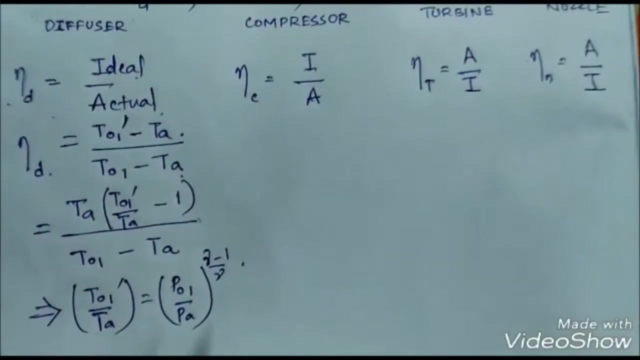 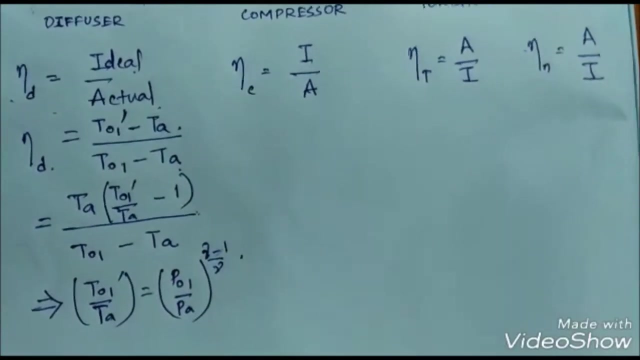 Now we know Now by isentropic relation, that is, T01 prime by TA equals to P01 by TA. gamma minus 1 by gamma. What is gamma? Gamma is an adiabatic constant. Gamma is an adiabatic constant. 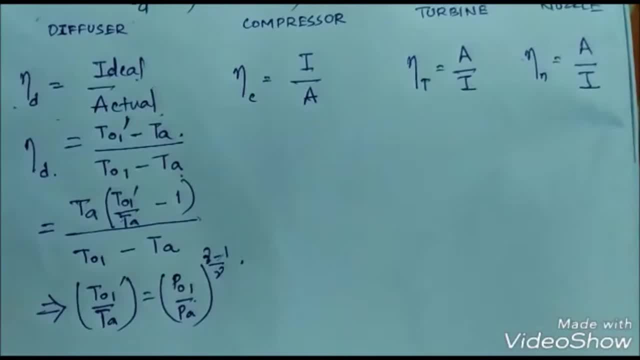 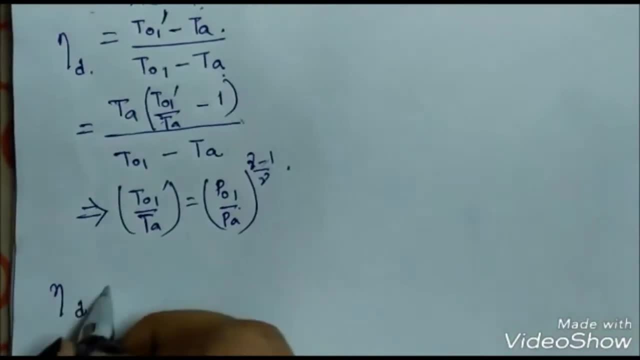 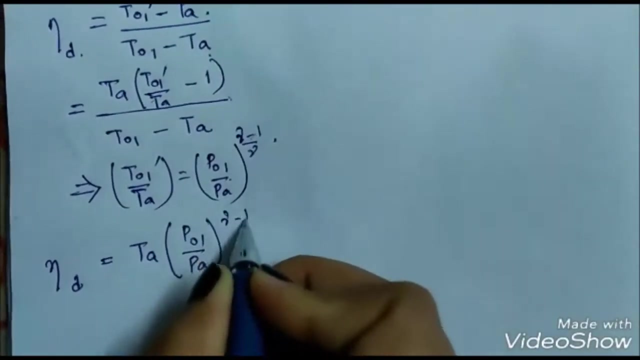 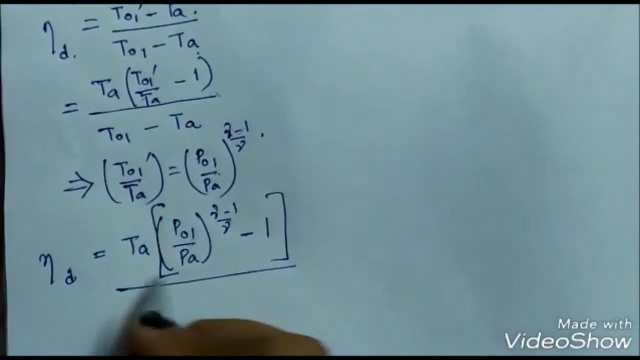 So now we are going to substitute this value in the above equation So eta D. So eta D equals to TA TA01 by PA gamma minus 1 by gamma minus of 1 divided by TA. let me take it common: TA01 by TA minus 1.. 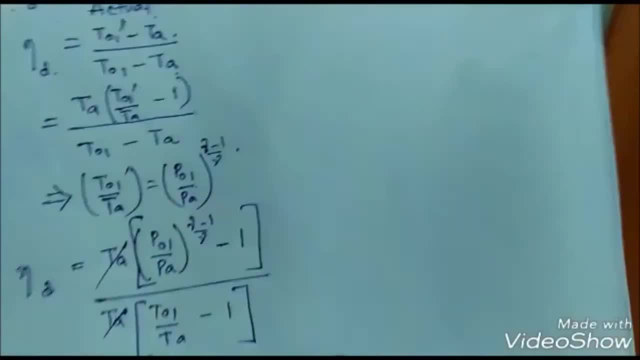 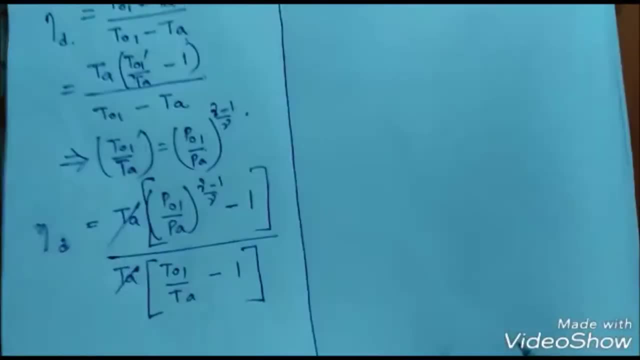 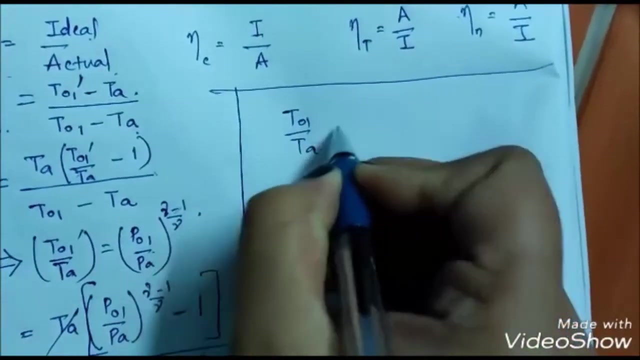 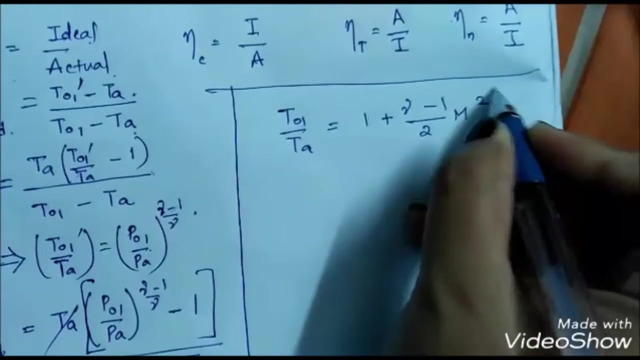 Let me cancel this TA, TA. Okay, Now how we can write this one, Okay. So also we know that you will be knowing that T01 by TA is equals to 1 plus gamma minus 1 by 2 M square. 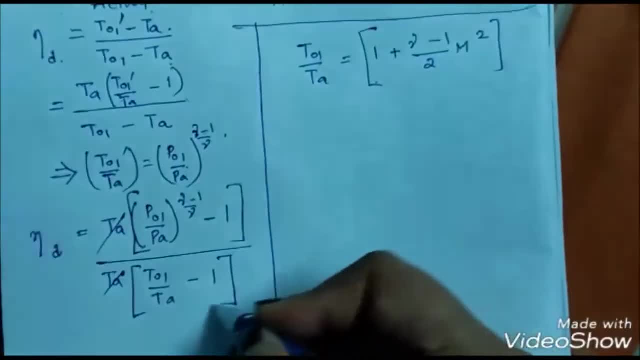 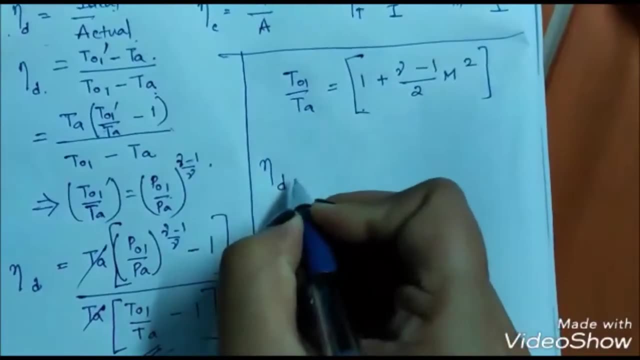 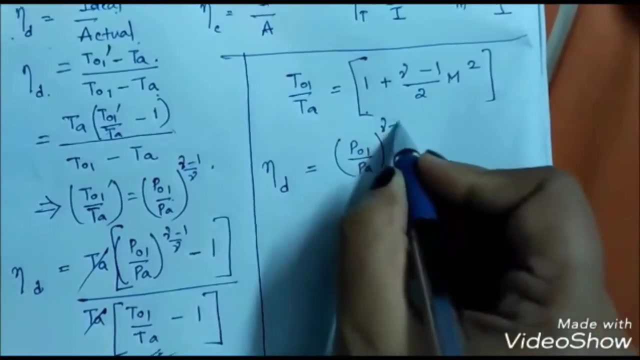 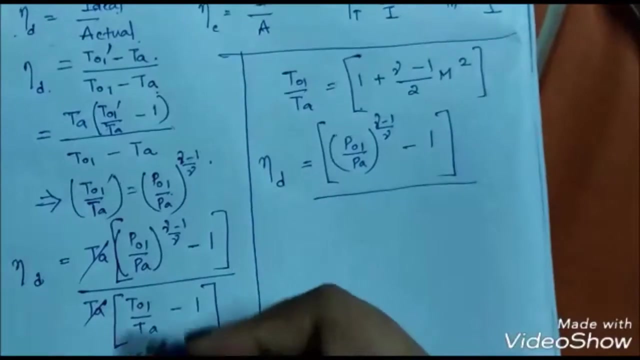 Right Now, again, we are going to substitute this value in this equation. Substitute this value in this equation. Let us see what happens. Eta D equals to P01 by PA gamma minus 1, by gamma minus 1 by. in place of this, we are going to substitute this value. 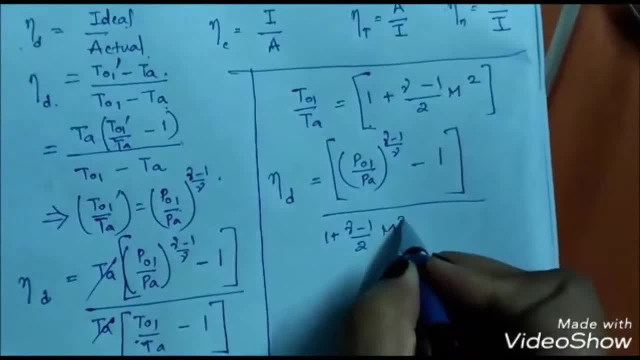 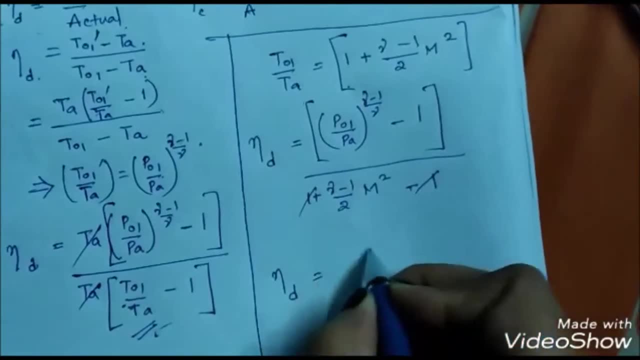 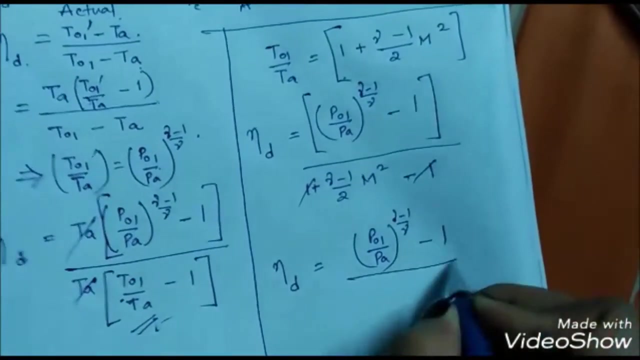 So 1 plus gamma minus 1 by 2 M square minus 1.. This minus 1 and this plus 1 will get cancelled. Eta D equals to P01 by PA. gamma minus 1 by gamma minus 1, gamma minus 1 by 2 M square. 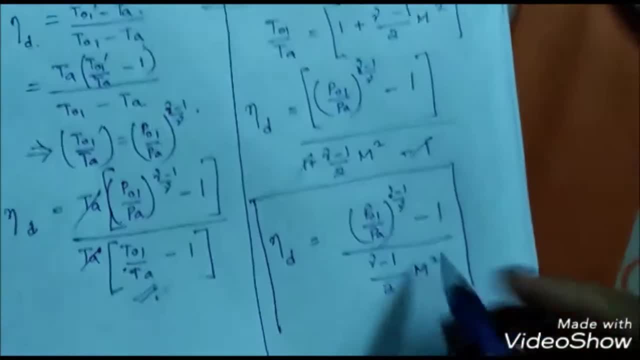 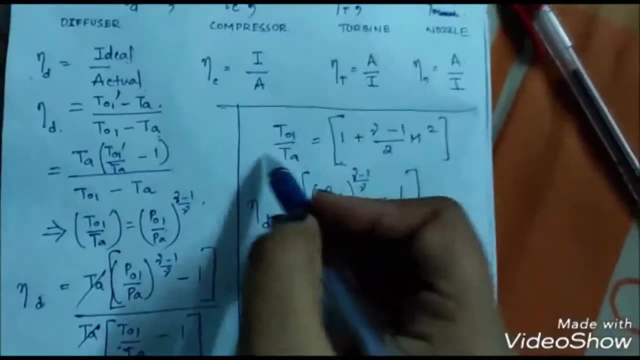 In some of the books you can find, they have directly given this formula to you, So you don't need to work so hard to remember this. Remember few of this small formulas. this one and this one, And you will get this. 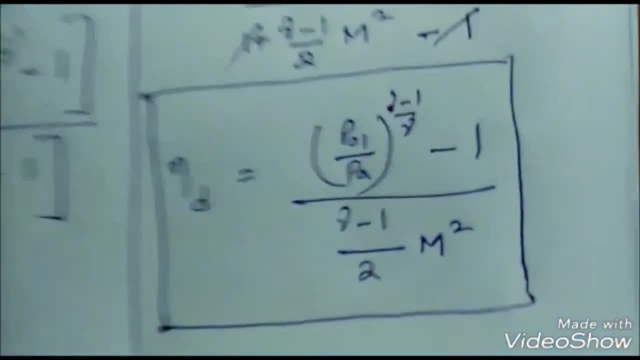 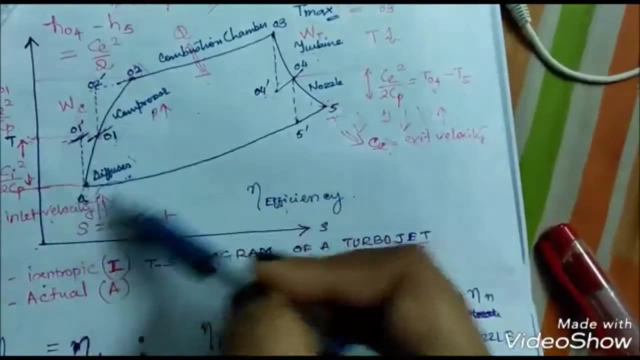 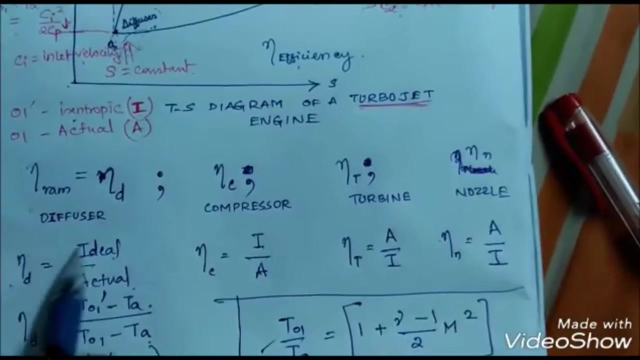 This formula Right on your hand. So you remember this technique, what I said, That is in this left hand side. what you have left hand side, all the formulas you are having that ideal by actual See this, these are the left hand side. 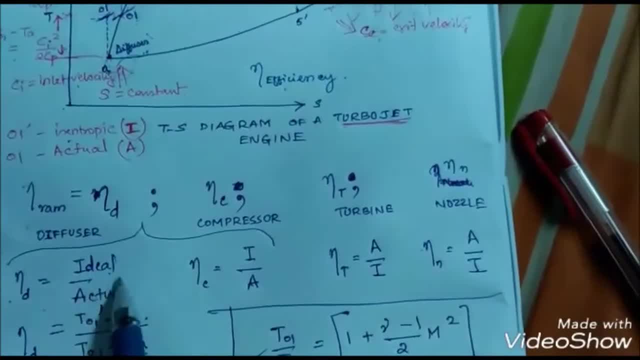 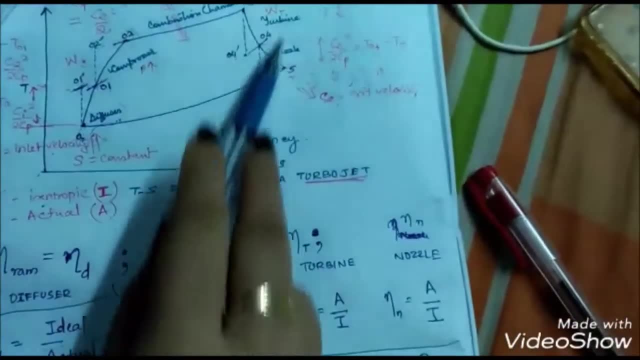 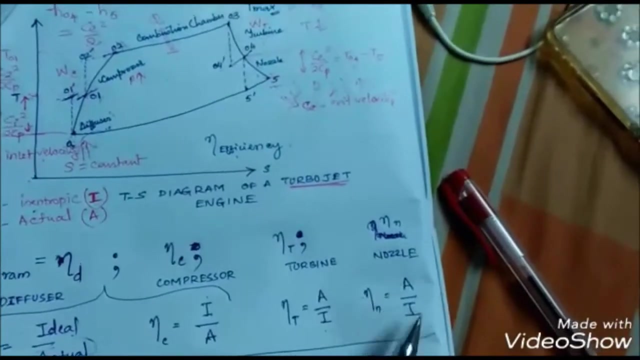 That is all. are I by A? So ideally you know what is the value and actually you know. So both the side we have ideal by actual, And the right hand side, you see that is turbine and nozzle. both we have an actual by ideal, actual by ideal. 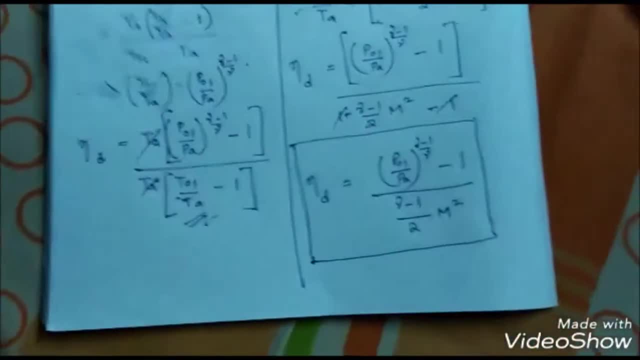 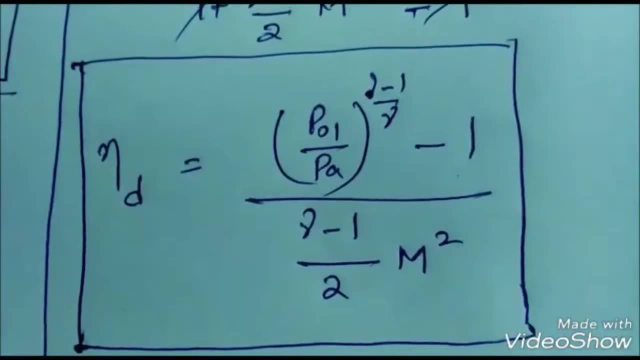 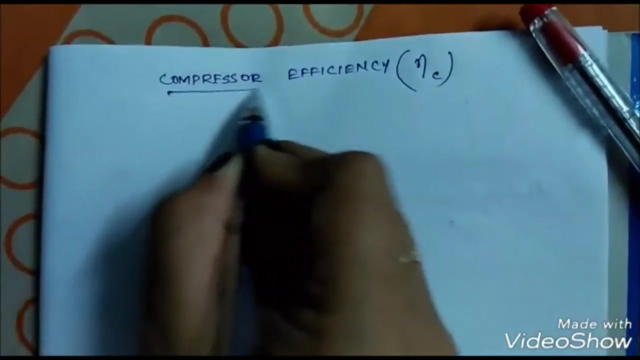 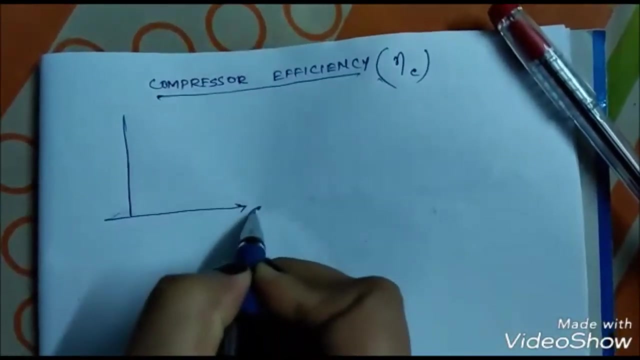 So remember that. and just like this diffuser equation, you can find this expression in a very easy way. Now we are gonna find the compressor. If you can see in the left hand side, there is no compressor efficiency, so we call the figure, that is TS. it's going like this from the point. 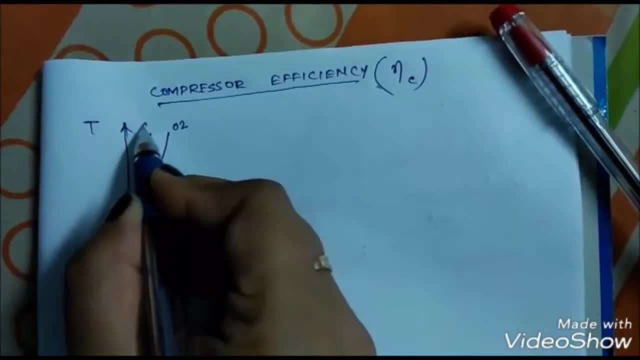 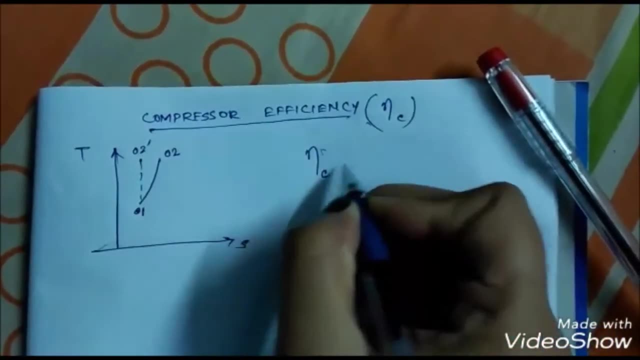 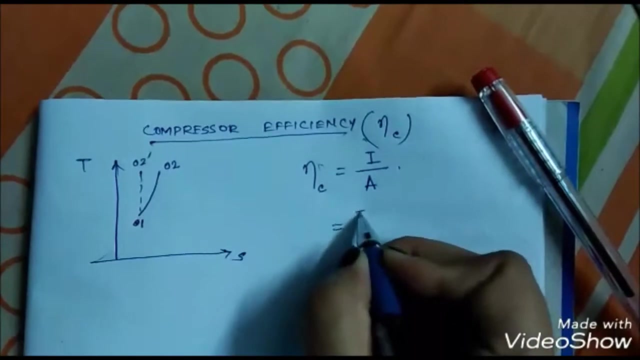 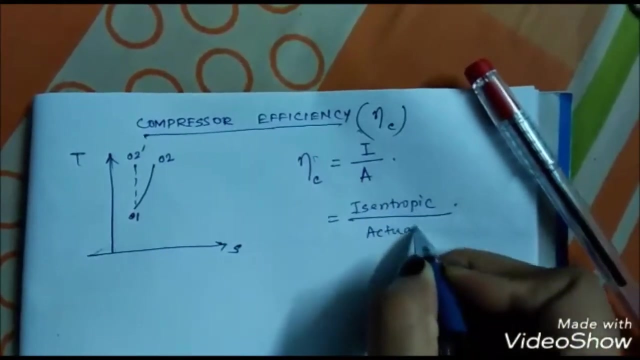 0, 1, 2, 0, 2- and this is a point- is 0, 2 dash okay. so what is a fundamental formula? I said eta C. eta C is what that is ideal by actual. so what is ideal? isentropic temperature divided by actual temperature difference. now let's 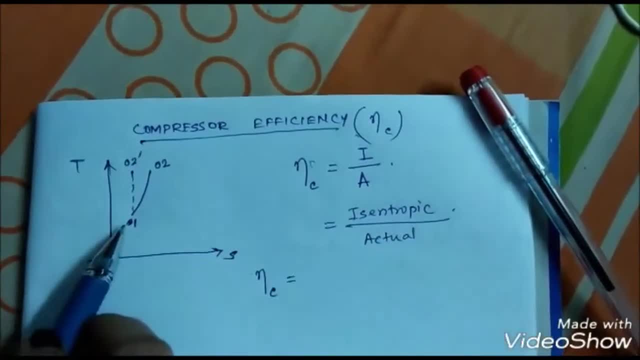 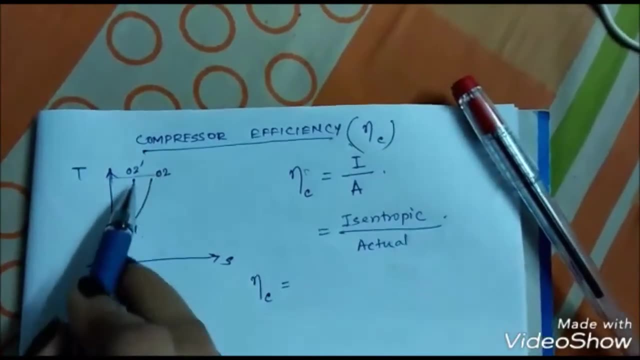 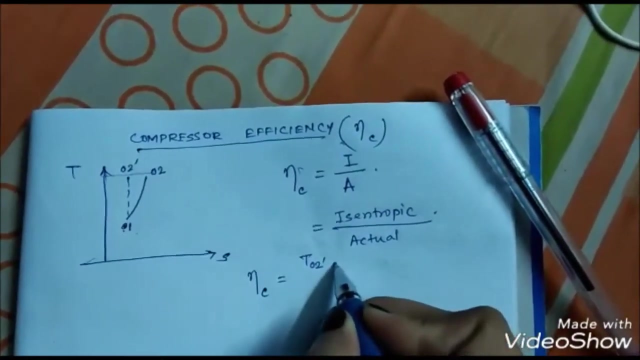 write it down what is isentropic? this is 0, 1, 2, 0, 2 dash. but who is in higher order, higher temperature? obviously 0, 2 dash. so right, 0 T, 0, 2 dash minus T, not 1 next. 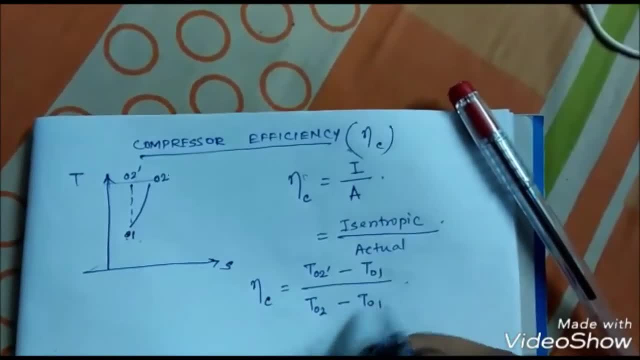 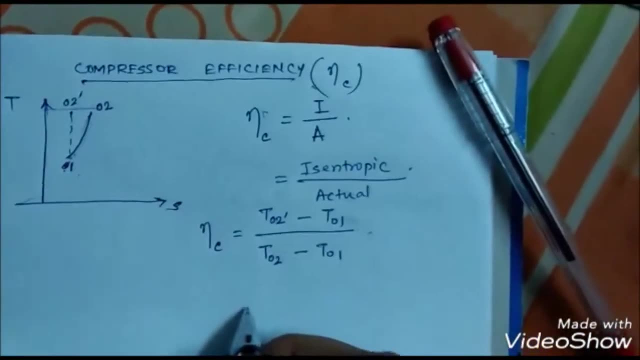 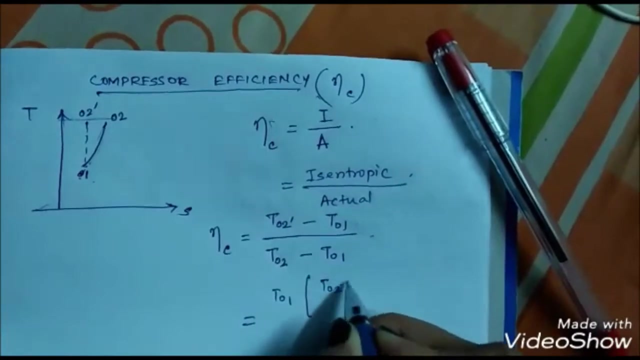 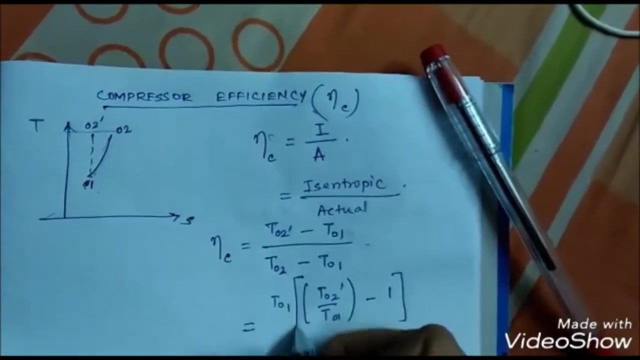 T not 2 minus T not 1, because this is our actual line, this is our ideal line or isentropic line. now, similar way, what we are gonna do, we are gonna take the T not 1, common T not 2 dash by T not 1 minus 1. 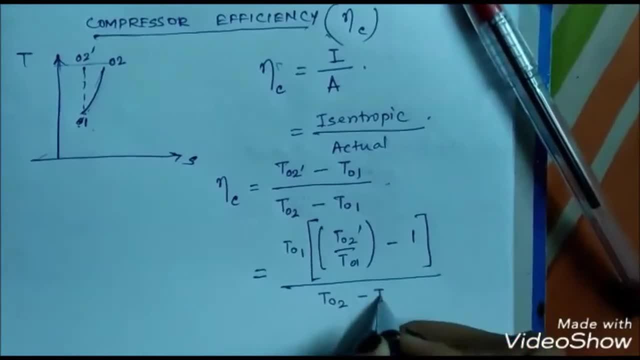 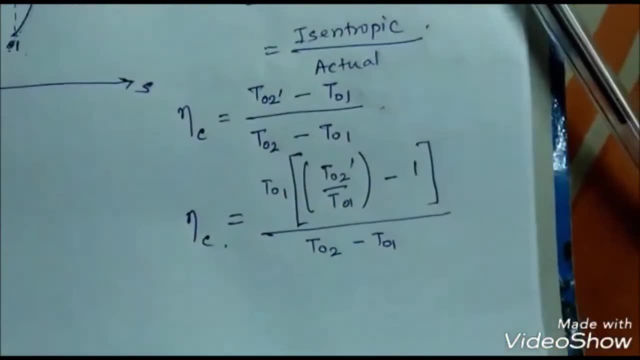 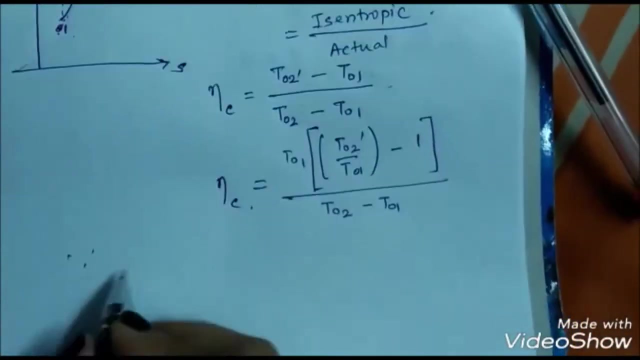 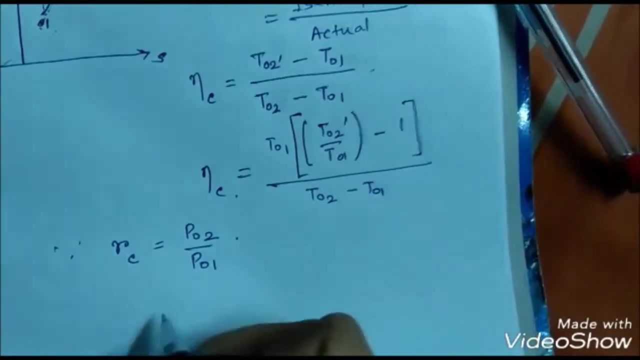 divided by. let this is be as. let it be like that. only to change this: equal to eta C. now, this is an compressor, so we know that there will be a a and as a compressor ratio. what is the compressor issue? P knot 2 by P knot 1. so 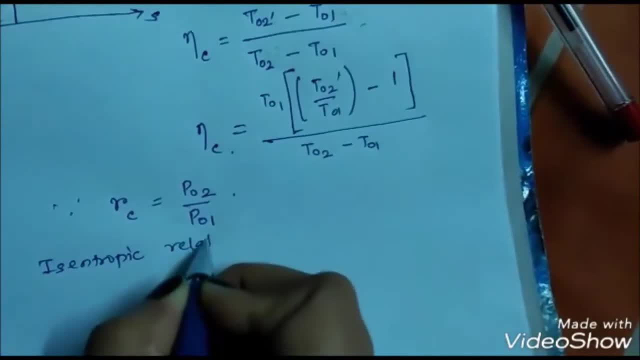 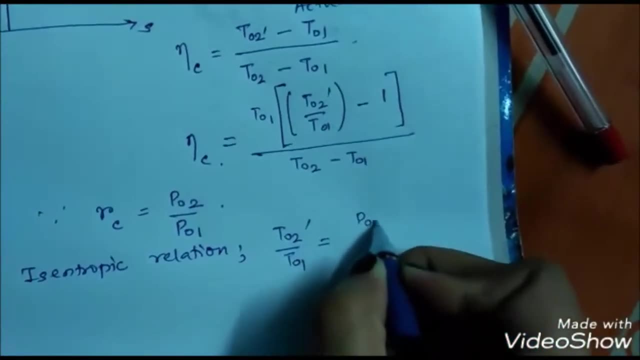 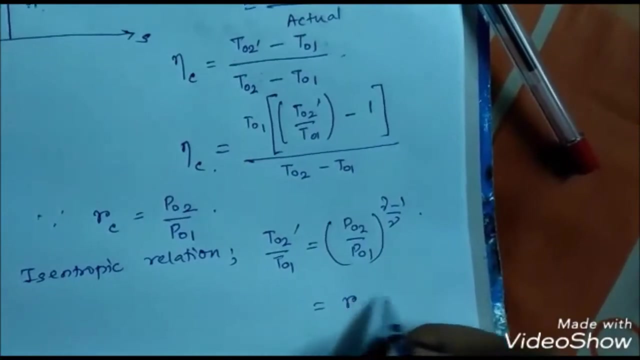 I sent Tropic relation again in isentropic relation, that is T not 2. dash by T not 1 is equal to P not 2, by P not 1. the gamma minus 1 by gamma, or rather we can say are see gamma minus 1 by T not one, by T not one. or we are see what. 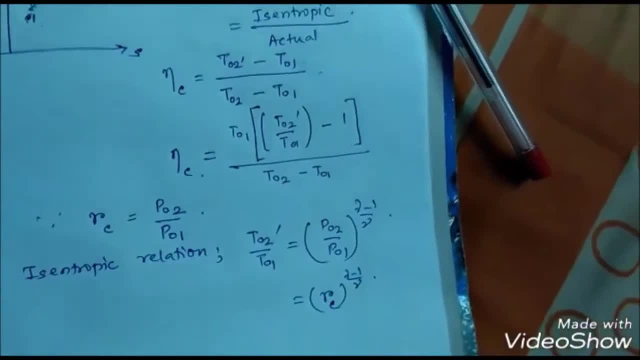 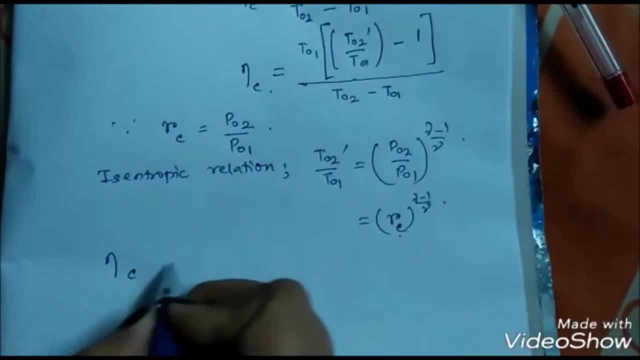 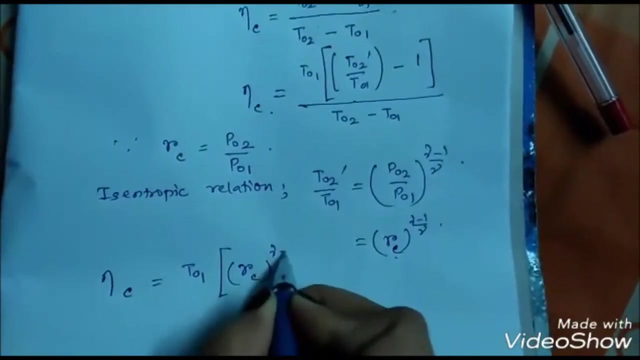 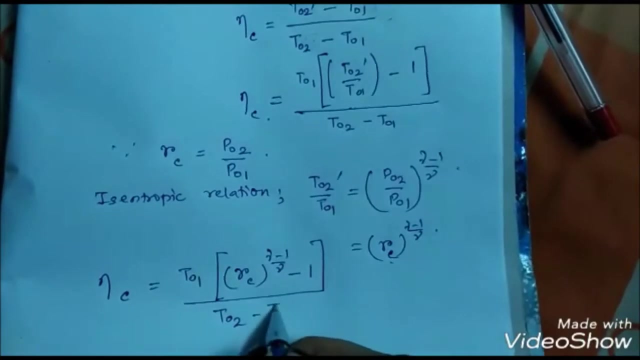 that is T not two by P. knot one has equal to P naught, twos by T, not one. we can see gamma minus 1 by gamma. Now this value we are going to substitute over there, Eta c equals to t naught 1 rc gamma minus 1 by gamma minus 1 by t naught 2 minus t naught 1. Is 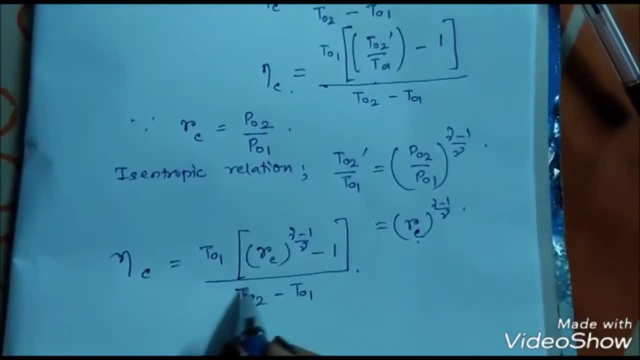 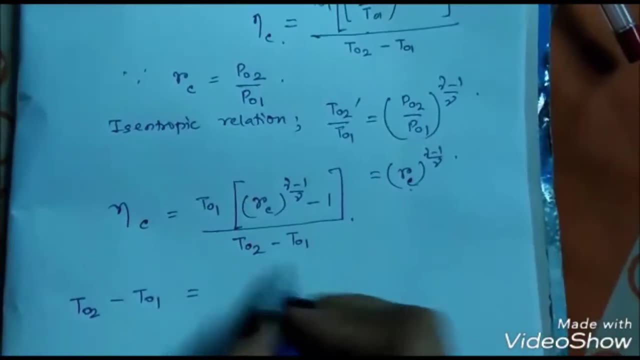 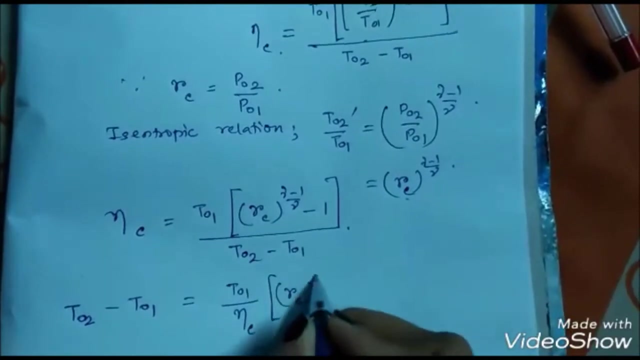 that clear. So usually in when you solve any problem, you need to find the t naught 2 minus t naught 1.. So how we can find t naught 1 by eta c rc gamma minus 1 by gamma minus 1.. 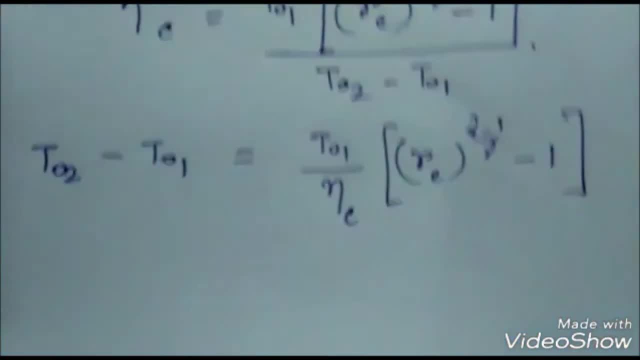 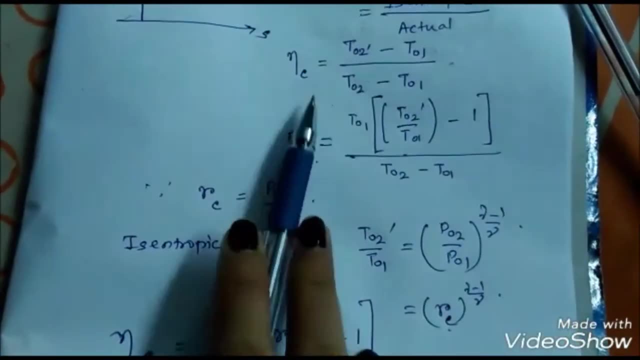 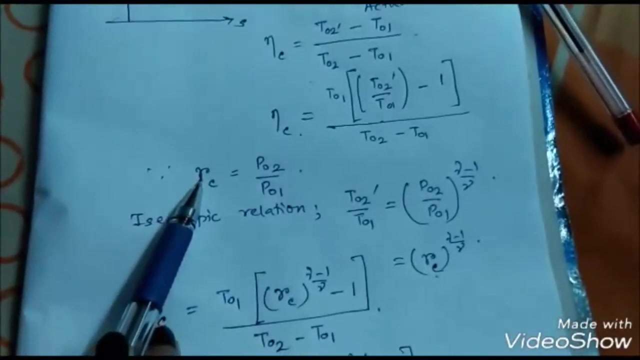 In some of the textbook you can see this formula has been given to you, So no need to worry about it. Remember the basic formula. This is a basic formula and you know how the procedures. What is the fundamental concept? That is, in compressor you will be having a p naught 2 by p naught 1.. That is a compression. 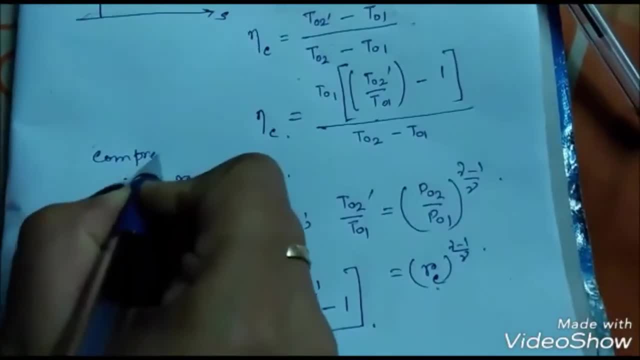 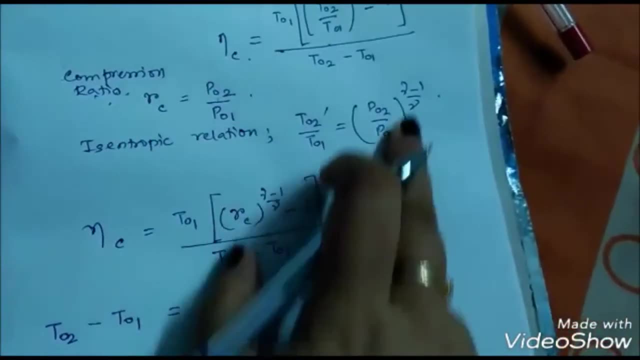 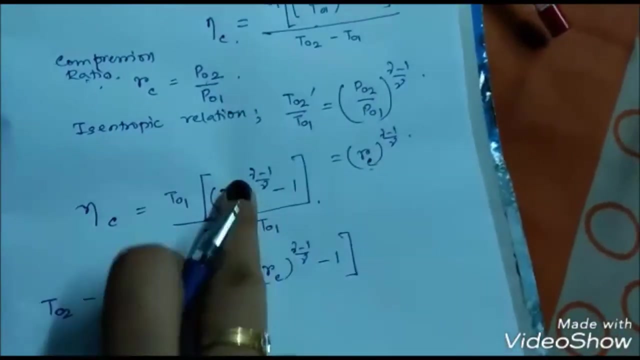 ratio. There is a compression ratio. Then, from isentropic relation, write this: Then what do you mean by p naught 2, by p naught 1?? That is rc. There is a p naught 2, and now we have made a Nik Привет number, So write 0.. 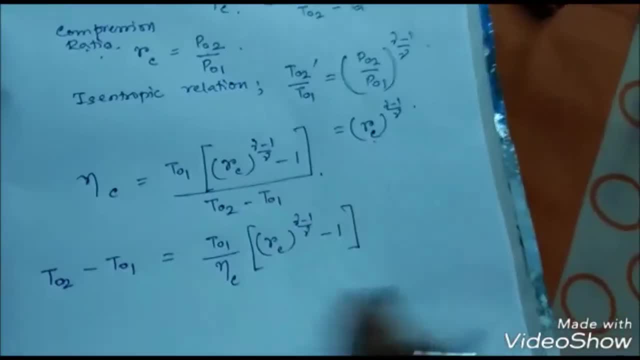 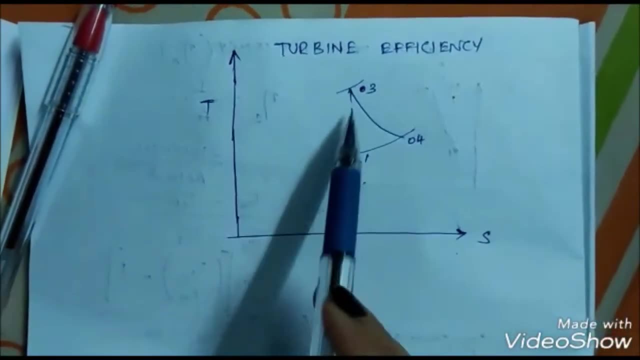 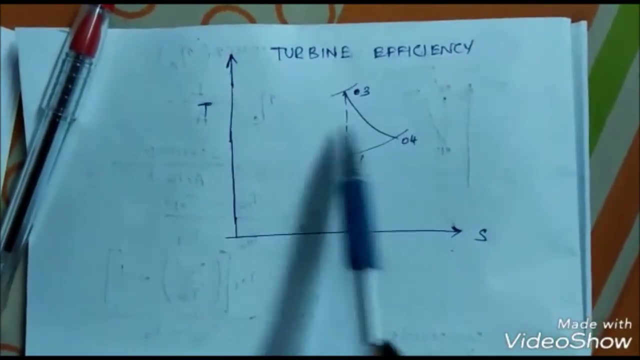 Then take the formula and substitute this: And what is the unknown value from this value? Then next we explain, Then you will get the expression. Now we are going to find the turbine efficiency. The turbine efficiency is the point between the zero three and the zero four. Thick line is an actual line and dotted line is an ideal. 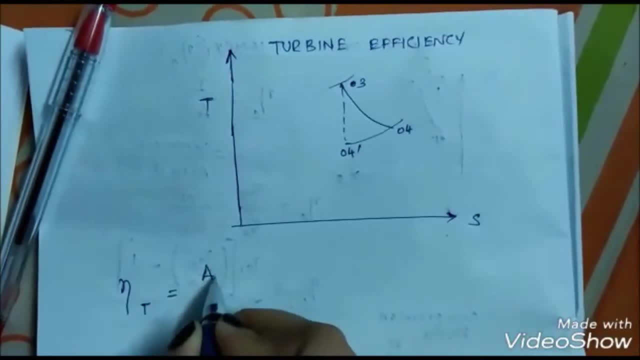 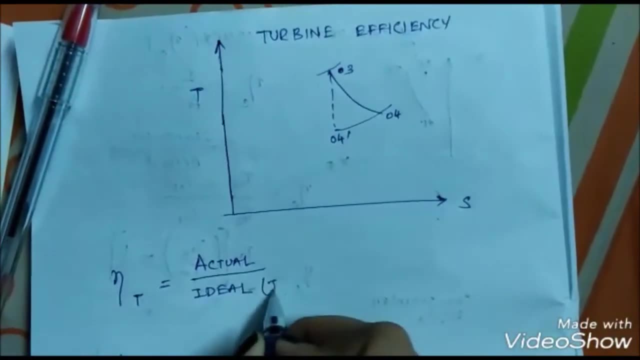 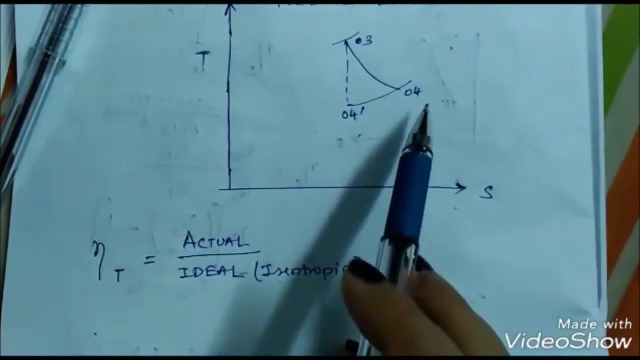 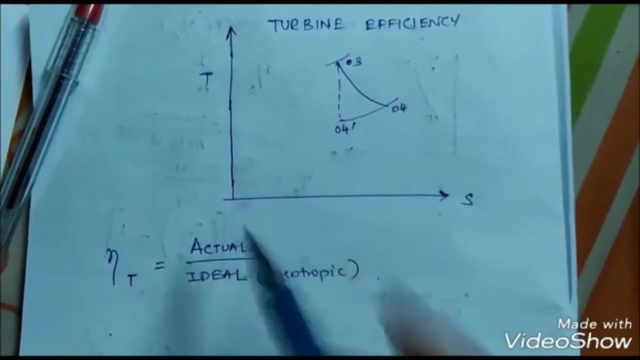 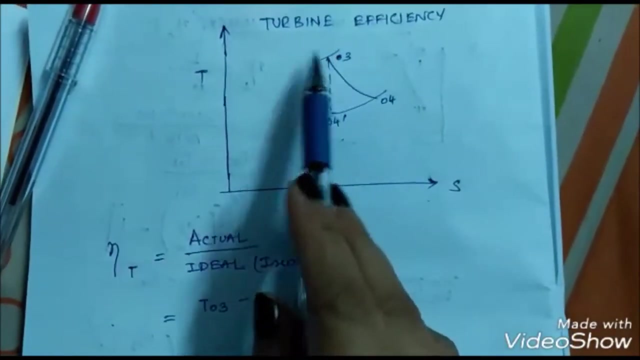 line. Now we are back to技术 by ideal or isentropic right. so here also we are going to write a relation between the t and the t, between these two points. so actual t naught 3, because the point 3 isn't higher compared to the. 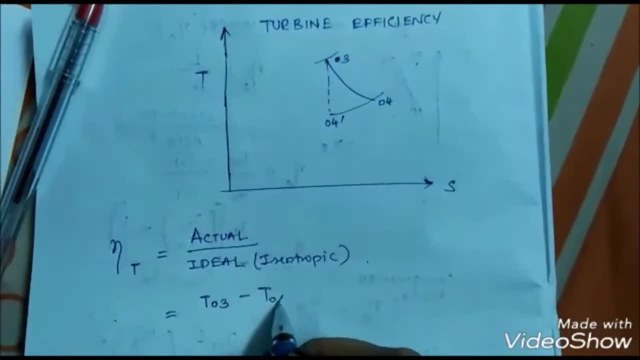 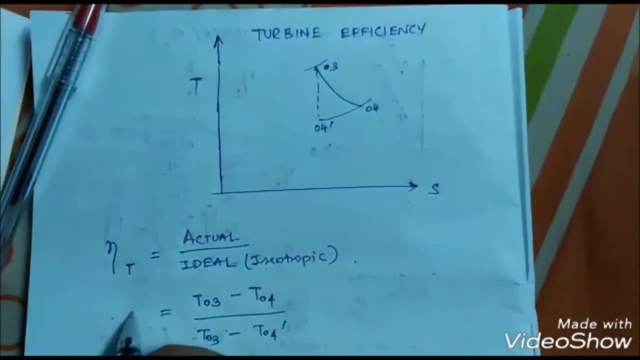 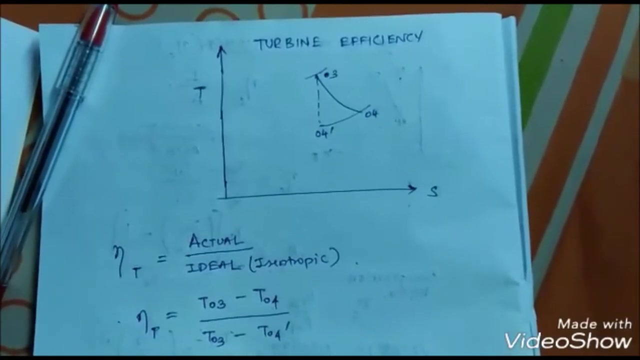 point 4. so t naught 3 minus t naught 4 by t naught 3 minus t naught 4, dash, so eta t okay. now, similarly here, t naught 3 minus t naught 4, divided by t naught 3, let's take it common, it is 1 minus t. 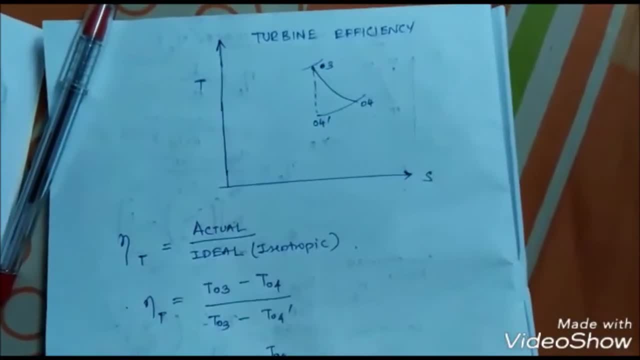 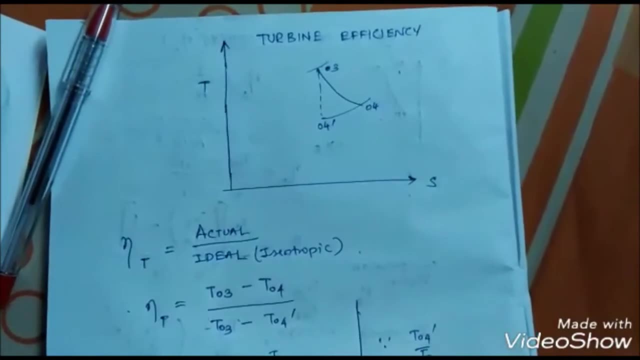 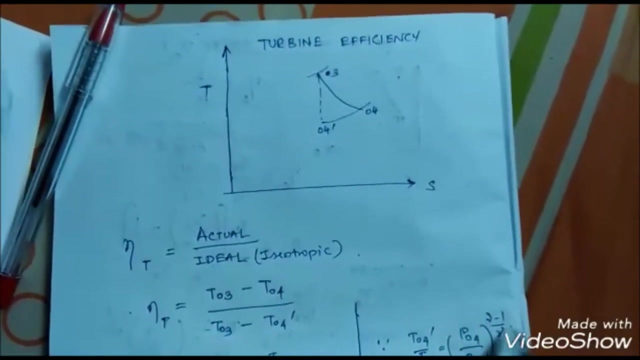 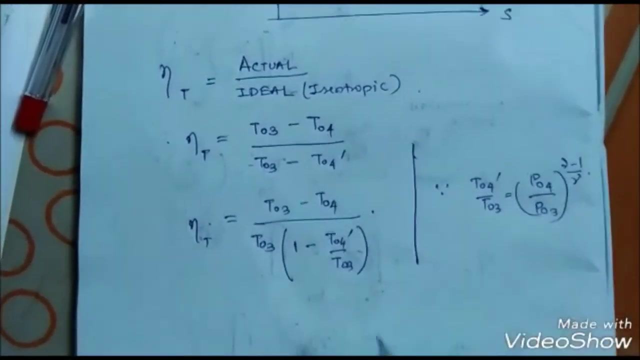 naught 4 dash by t naught 3. so we know that t naught 4 dash by t naught 3 equals to p naught 4 by p naught 3. gamma minus 1 by gamma, gamma minus 1 by gamma. so we are going to apply it over here. 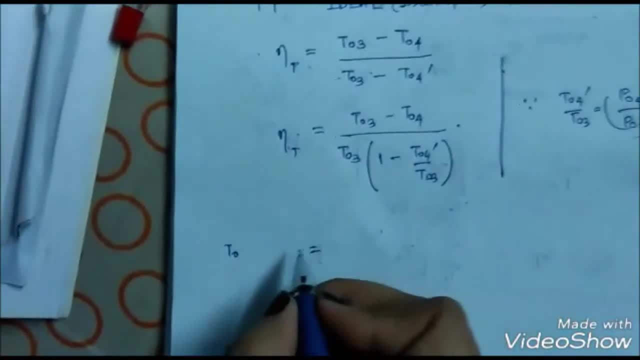 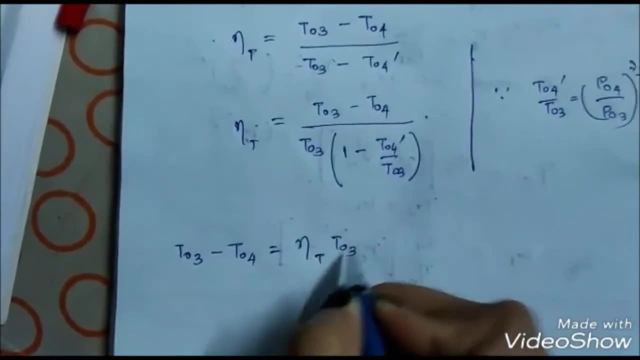 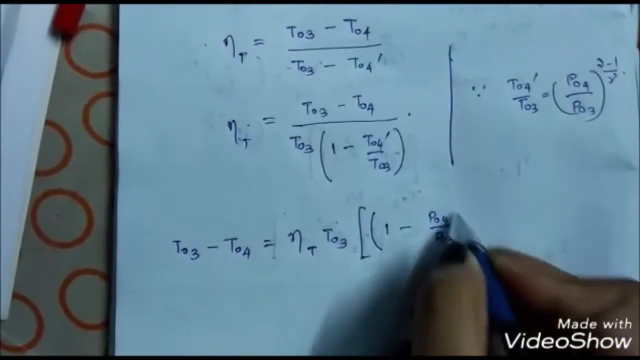 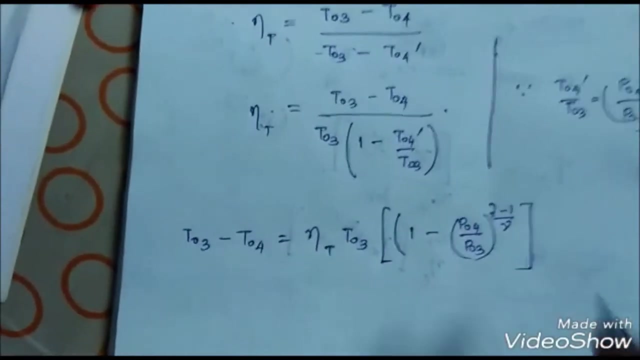 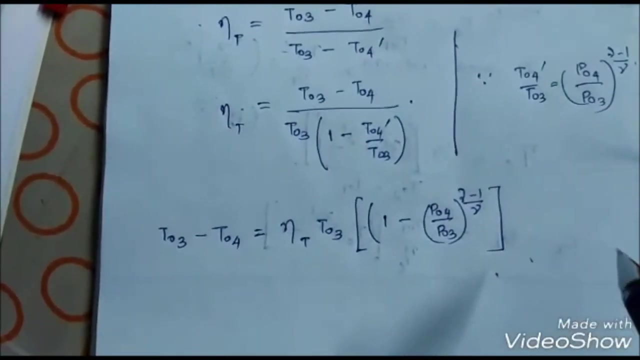 we can write then. overall we can write like this: t naught 3 minus t naught 4, eta t in the bracket 1 minus p naught 4 by p naught 3, gamma minus 1 by. this is one of the expression to find this relation. now, 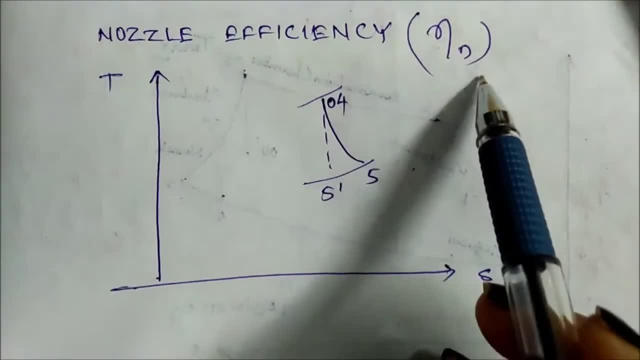 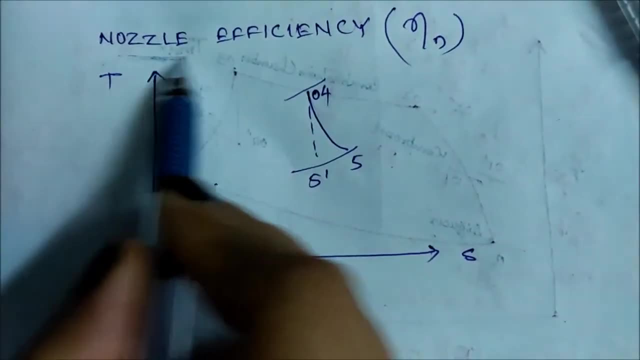 we are going to see a nozzle efficiency that is eta n. so this is a table头, that is, we can write here to find the this relation equation. now we are going to see our nozzle efficiency, that is eta n. so this is a t is diagram for nozzle nozzle. what is the purpose of nozzle? to increase the velocity. 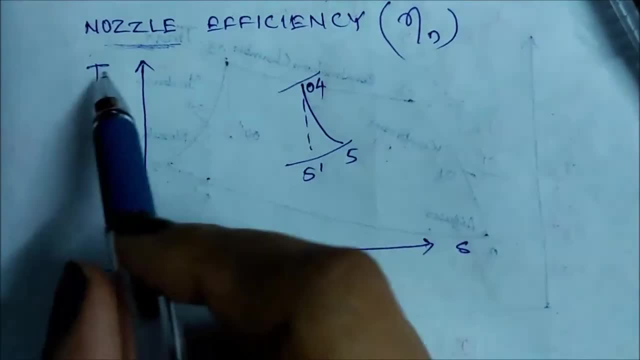 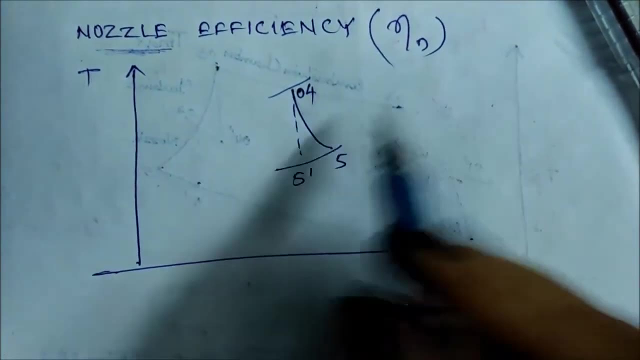 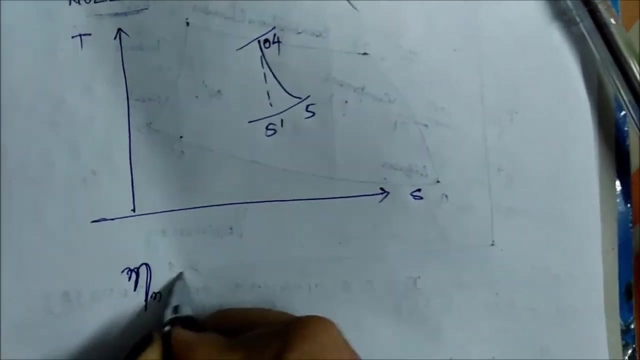 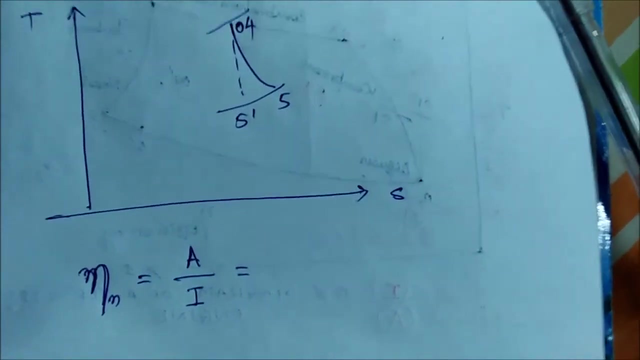 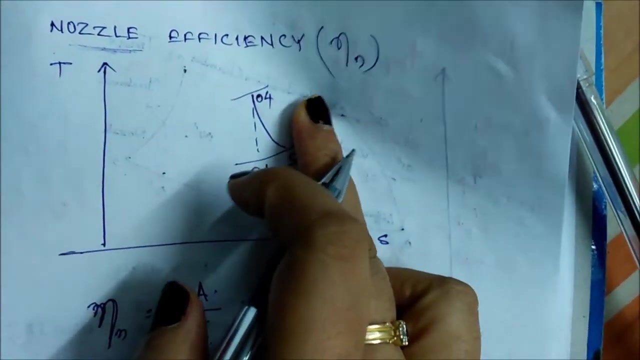 so increase the velocity, pressure will decrease and the temperature will also decrease, because pressure and the velocity are inversely proportional to each other. now what we have studied, what is nozzle efficiency? that is actual, by ideal or isentropic form. so now we are going to write a temperature in between the actual and the ideal. so who is having the highest? 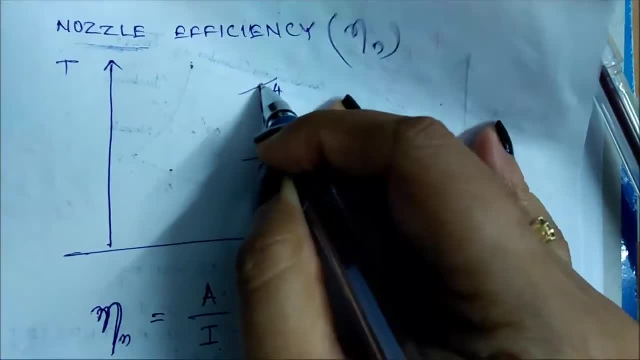 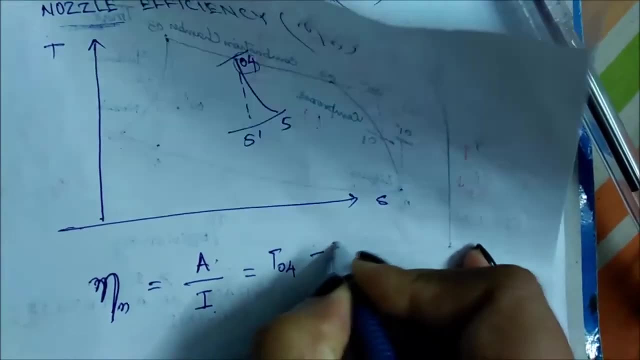 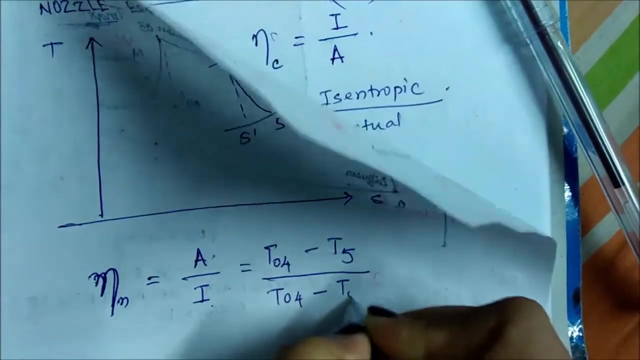 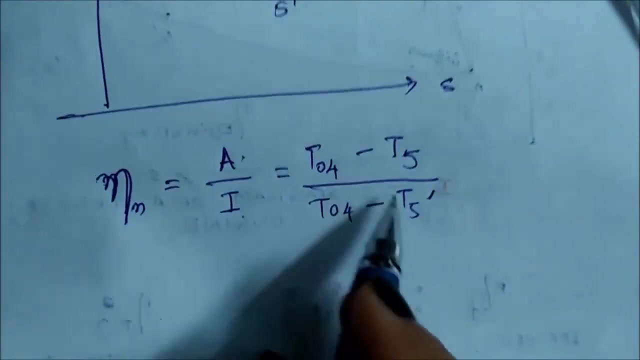 temperature high. that is 4 compared to the 5. so first we'll write t naught 4 minus t naught minus T5, divided by T04 minus T5. dash right, okay now. what we are going to do now, same as the. 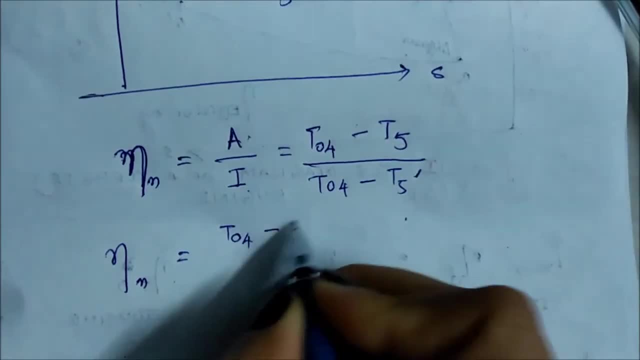 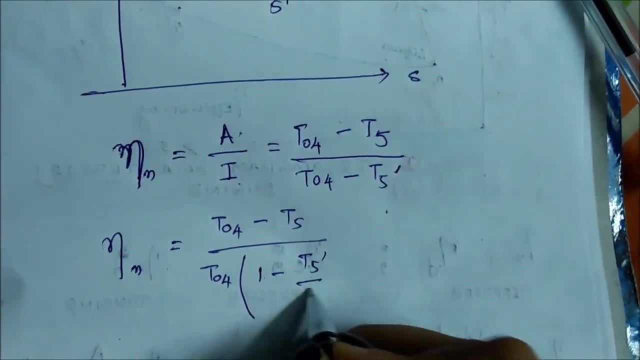 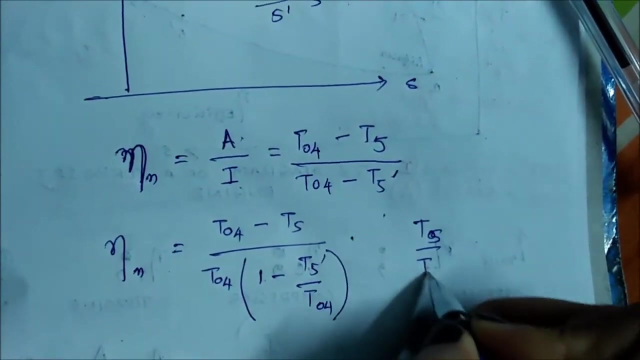 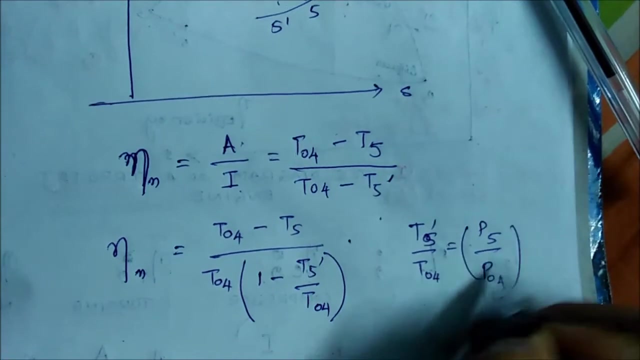 other one. we are going to take the T04 outside. we are going to take the T04 outside. so 1 minus T5 dash by T04, okay, now, what is T5 by T04, it is P5 by P04, gamma minus 1 by gamma. 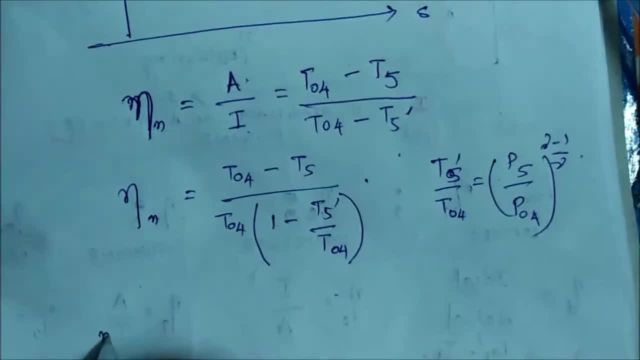 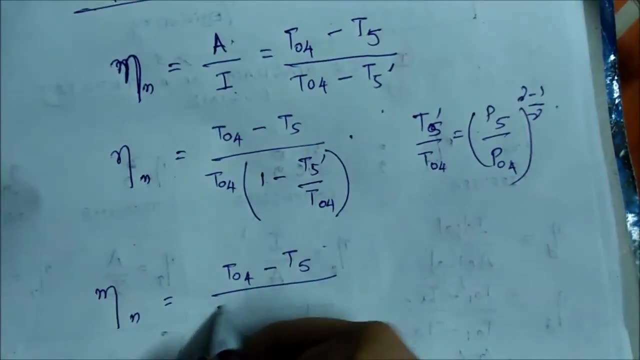 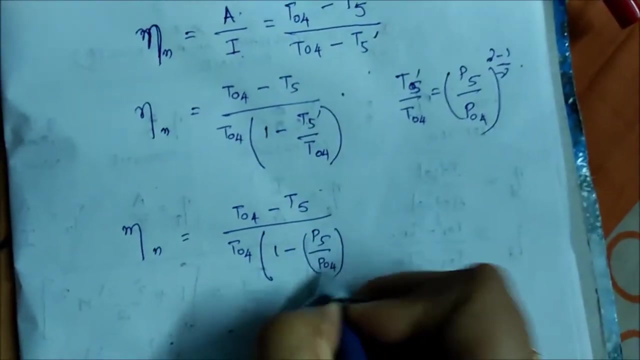 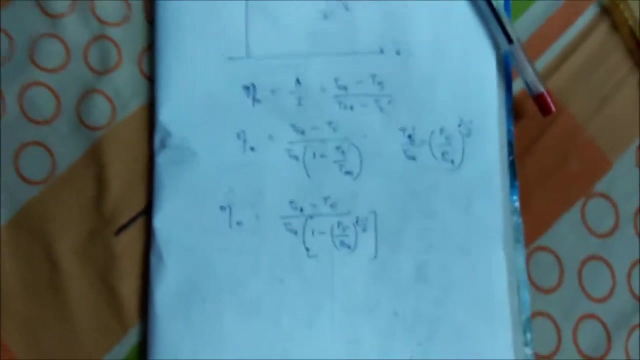 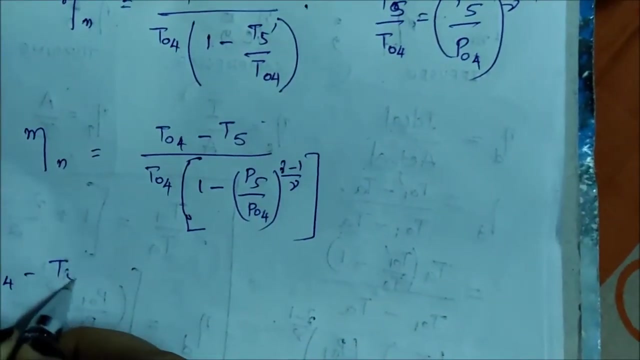 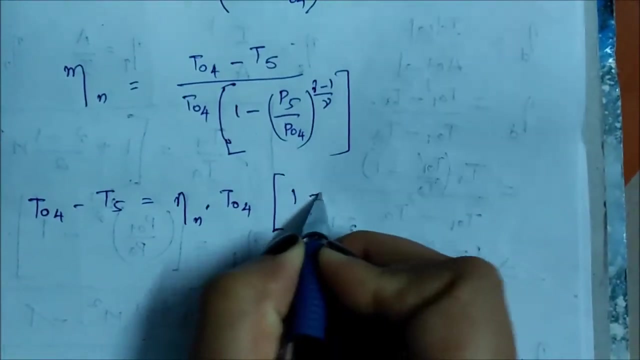 now this value we are going to substitute over here. okay, eta n. T04 by T5 by T04, this 1 minus P5 by P04 by gamma minus 1 by gamma. close the bracket. okay now, using this relation, P04 minus P05 equals to eta n into T04, 1 minus P5, P04 by T04, okay now. 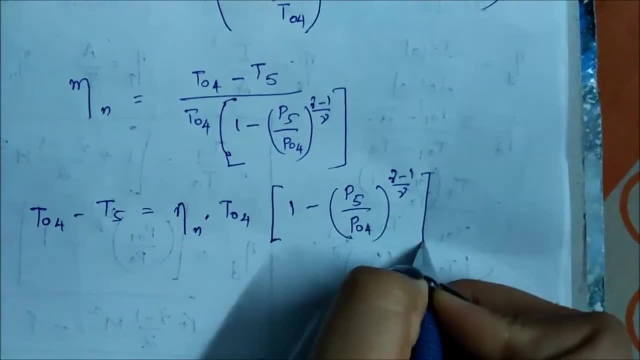 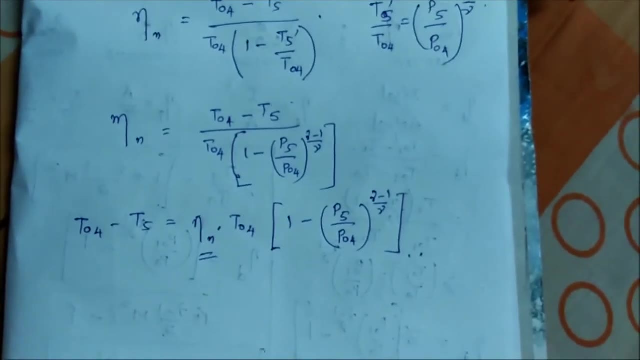 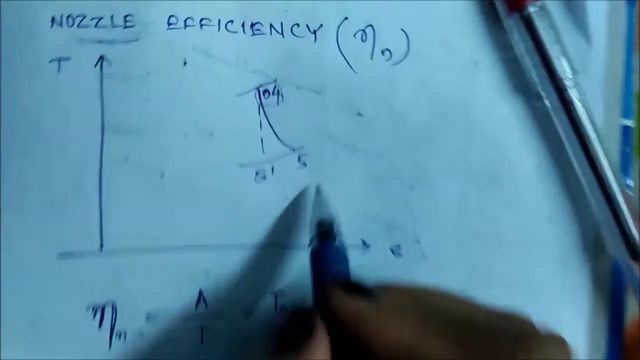 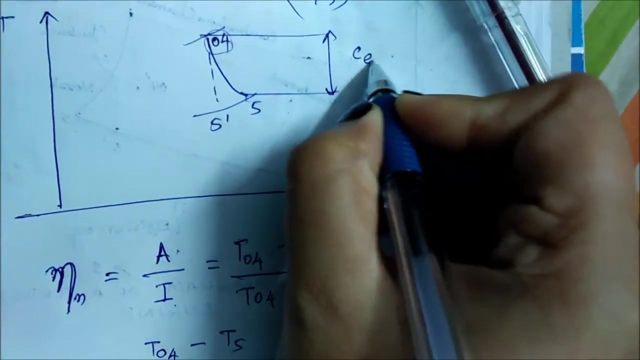 this is the expression for the nozzle, that's for the given data and the given requirements we can write. so we also know another thing: that is T04 minus T05, that is a this distance between these two. what we have said in the first one, that is, it is a CE square by 2. 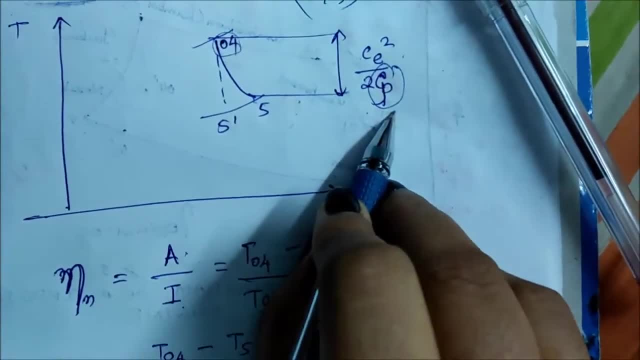 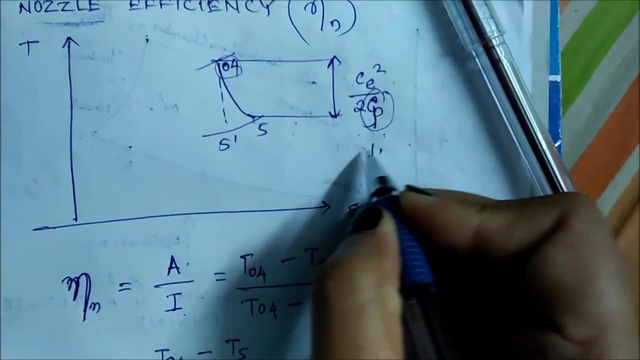 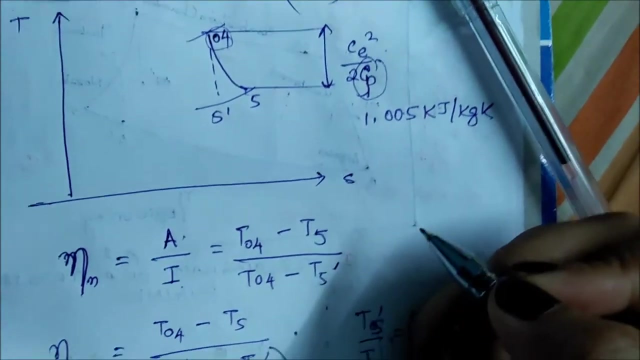 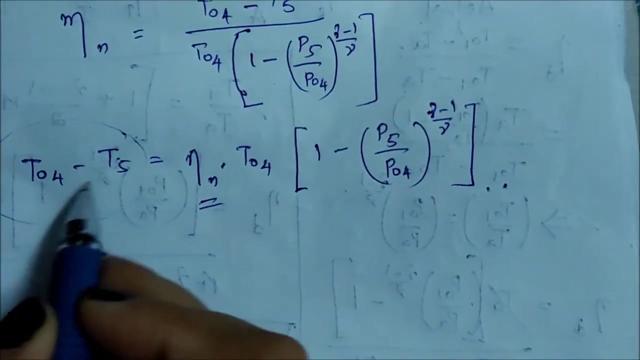 Cp. what is Cp is a specific heat at constant pressure. specific heat at constant pressure. we usually consider 1.005 kilojoule per kg kelvin. kilojoule per kg kelvin. so we, instead of this, that is C04 by minus C05, we can also write CE square by 2 Cp. okay, so we. 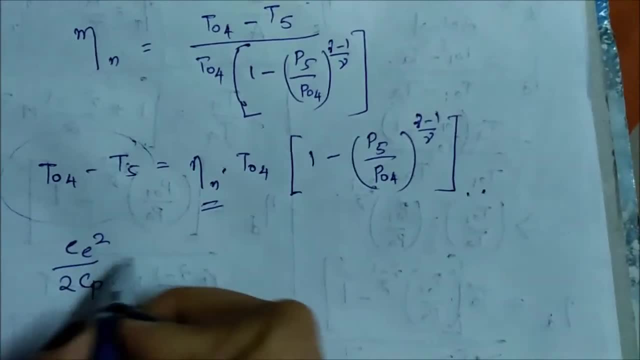 can write CE square by 2 Cp. okay, so we can also write CE square by 2 Cp. okay, so we can write CE square by 2 Cp. equals to eta n. T04, 1 minus P5 by P04, gamma minus 1 by.